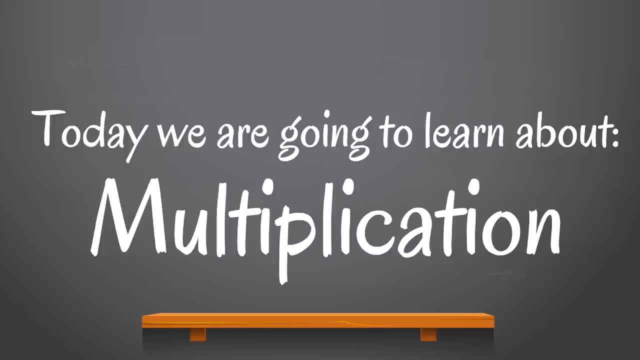 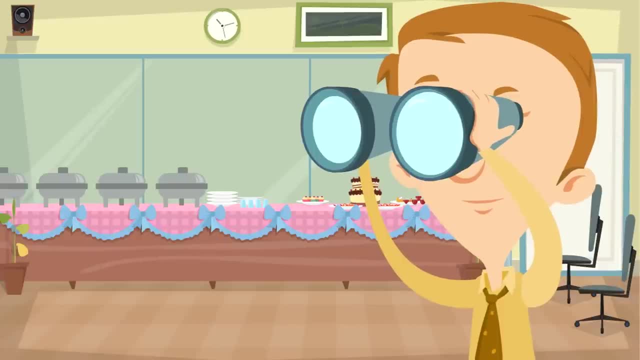 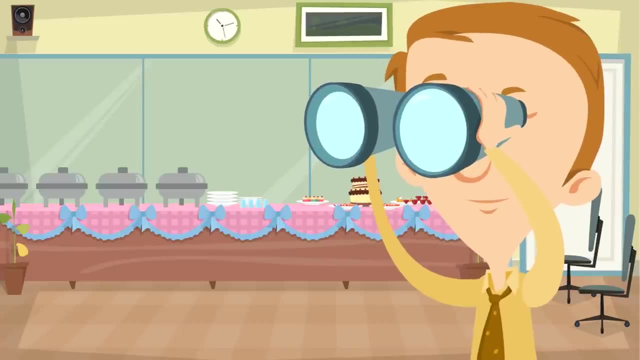 thing, it's just because you don't know how to do it. yet. Once you learn the game, once you learn the process, it's fun, it's awesome. You see, multiplying is like being a detective: You're cracking a code, which is so cool. You're solving mysteries like legit mysteries, Like. 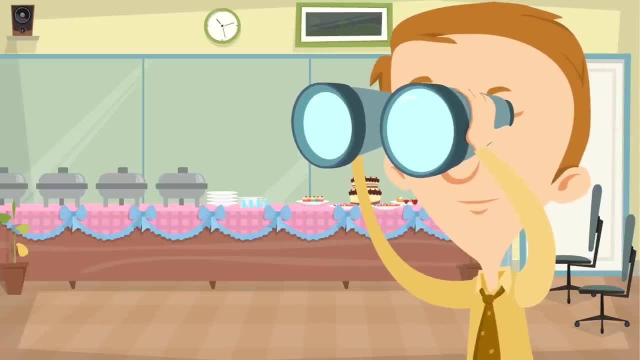 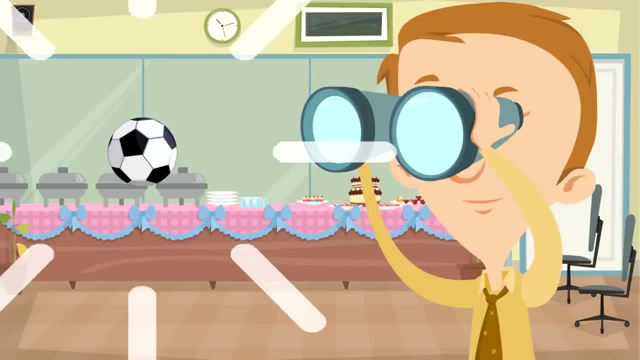 I'm in an office building right now. there's a cake behind me, For some reason. I'm looking out right now at you guys and I see that you're like, wow, we're going to multiply, And once you learn it, it's just a game. so buckle in for the fun and the learning. 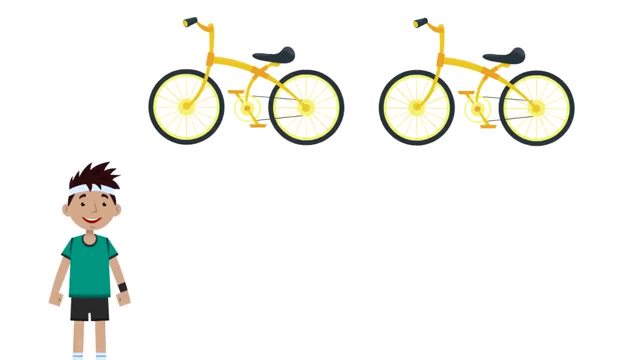 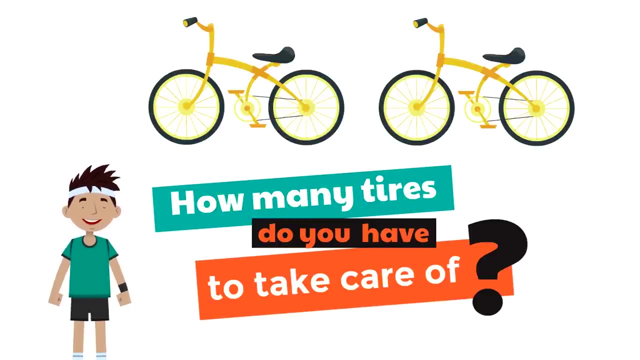 Let's say you have two bikes and for some reason they look the exact same and somebody wants to give you an air pump. They ask a simple question: How many tires do you have to take care of? To figure that out, we're going to use multiplication. We're going to 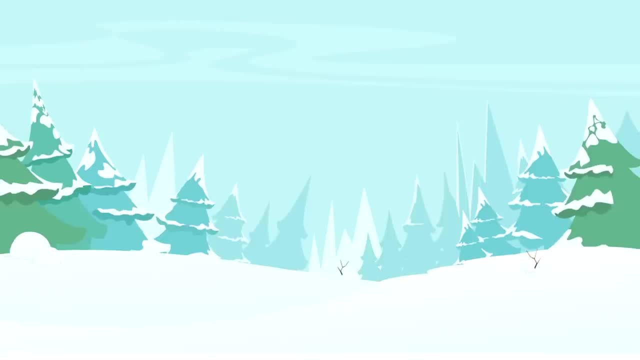 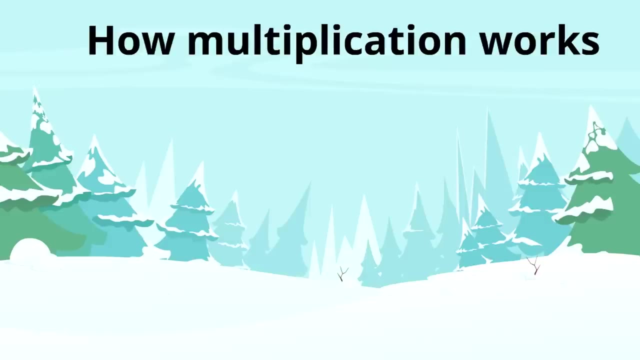 play the game. It's going to be awesome. Okay, so here is how multiplication works. Okay, so here is how multiplication works. Okay, so here is how multiplication works. So we put the number that's in each group and then we put this X, which means times, and 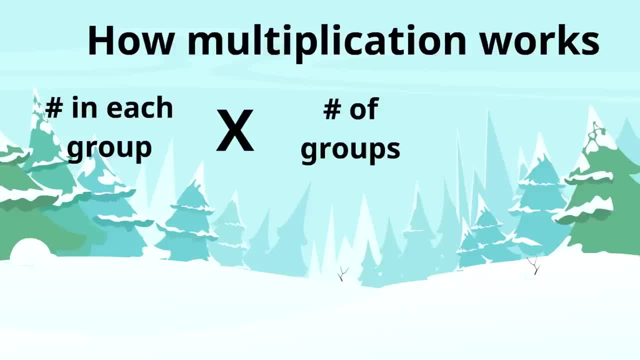 then the number of groups. So that tells us how many times that number is going to show up, and then we add them all together and you've got your answer. Isn't that cool? And just a side note: to work there has to be the same number in each group. Now, remember, we're 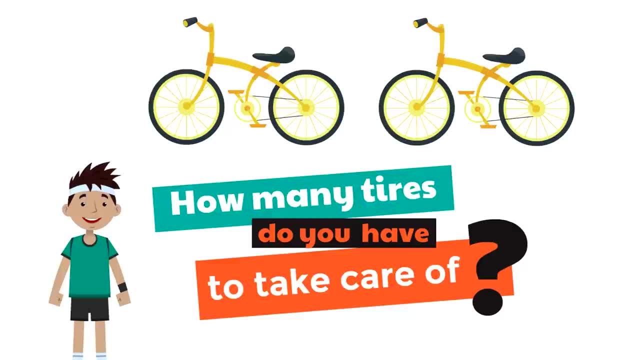 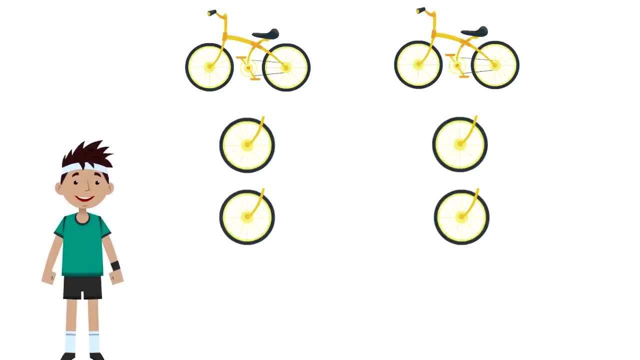 going to figure out how many tires you have to take care of if you have two bicycles. All right, now we have the wheels under each bike. Each bike has two wheels, One, two. So we write down a two. Each bike has two wheels. Remember the first number we write down with? 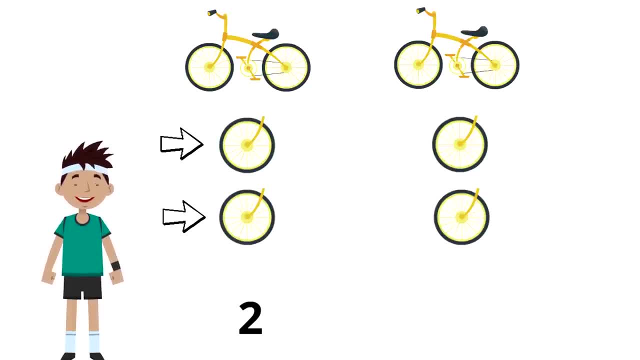 is the number in each group. Then we write an X. This X means times, Two, times. It's the symbol of multiplication. All right, the second number we write are the number of groups. You can see them here. How many groups do we have of two? How many? Yeah, two, So it. 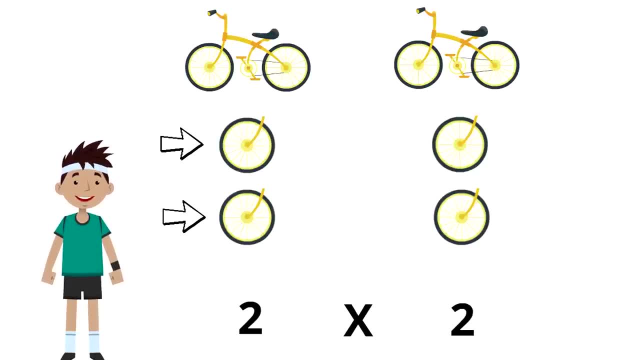 means two times two. To figure this out, we are going to skip count by two, Two, four. That means two times two equals four. If you have two bikes, that means you have four wheels. Two two times is four. 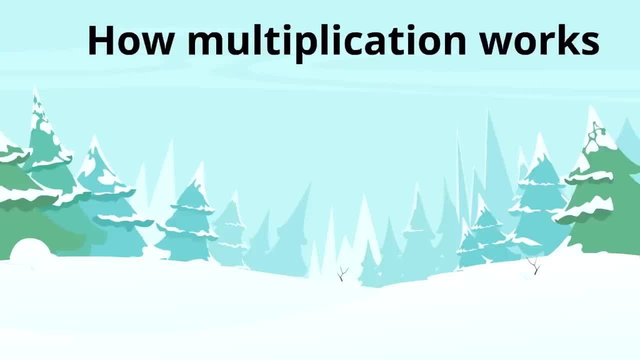 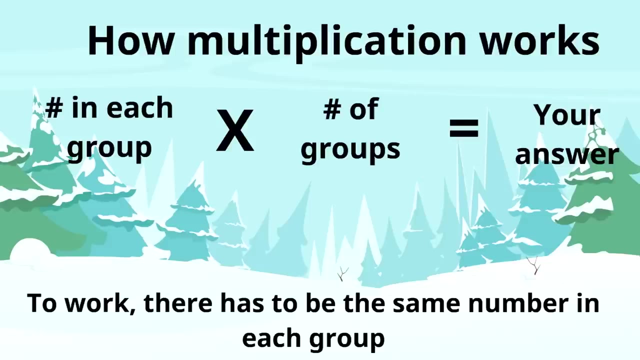 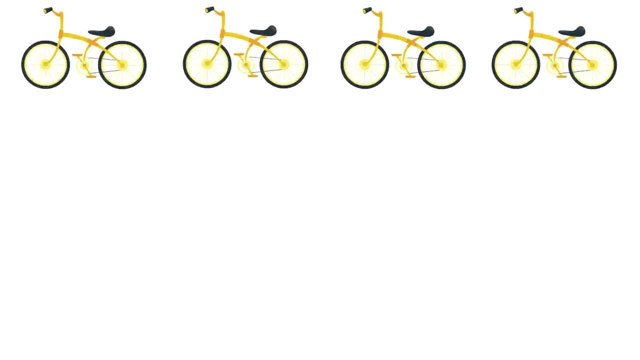 Remember. this is how multiplication works. The number in each group times the number of groups equals your answer. Of course, to work there has to be the same number in each group. All right, let's take this to the next level. Let's say someone has four bikes And 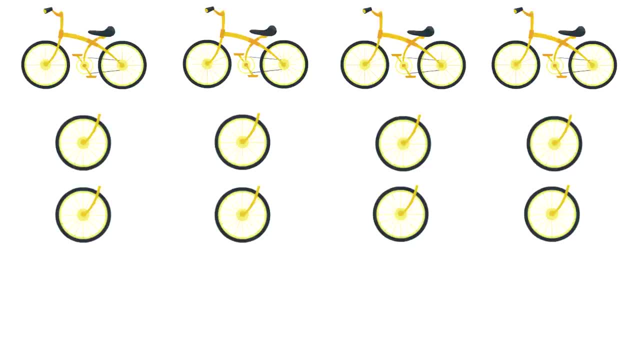 here are their wheels. Woohoo, Yeah, You know how to do this now. Each bike has two wheels, So the first number we write down is the number two. That's the number in each group We're going to put the time symbol. 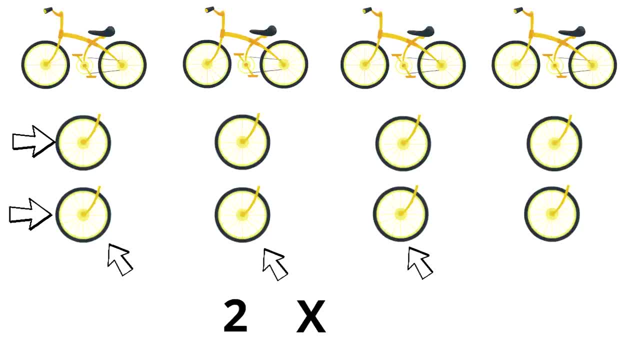 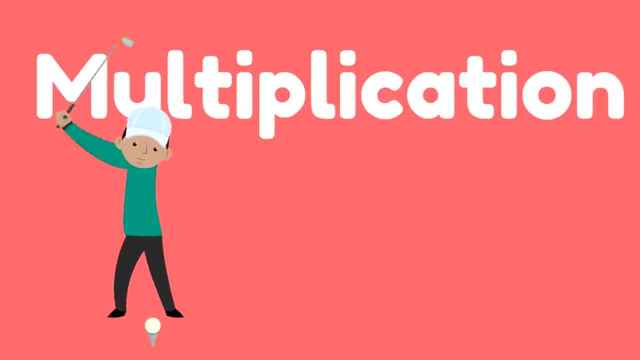 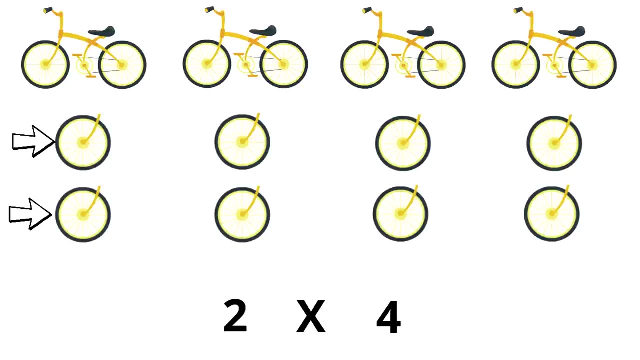 there and count the number of groups: One, two, three, four. So it's two times four. This is so much fun. This is multiplication. Now let's skip count to get the answer. Two, four, six, eight. Eight is our answer. 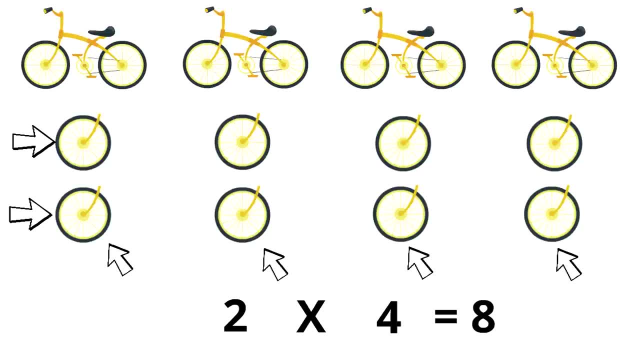 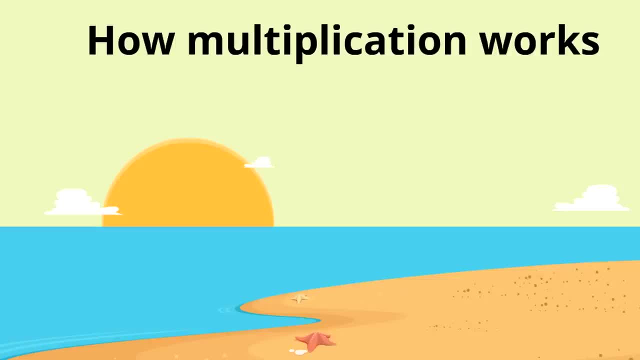 There are eight wheels. Two times four equals eight. This is how multiplication works. We put the number in each group times the number of groups and we get our answer. You're getting the hang of it. Subtitles by the Amaraorg community. 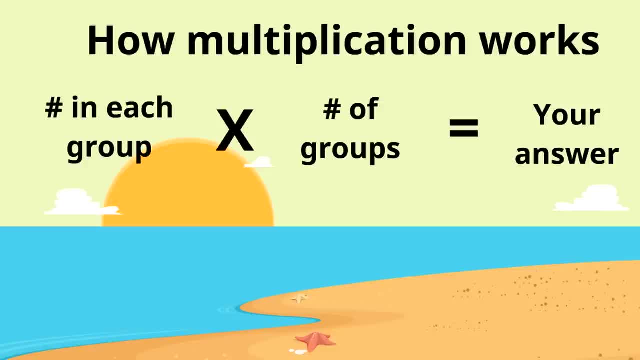 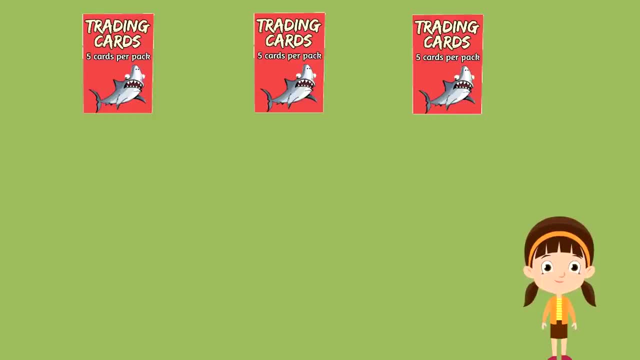 alright, let's try this one. let's say you buy three packs of trading cards. let's say each pack had five cards in it. huh, that's pretty good amount. so three packs of five cards, how many cards did you get in total? it's a really great question. 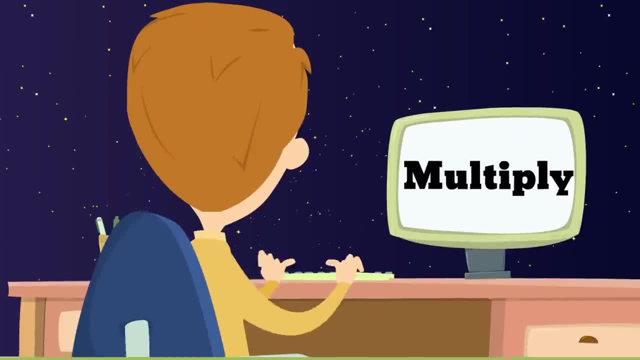 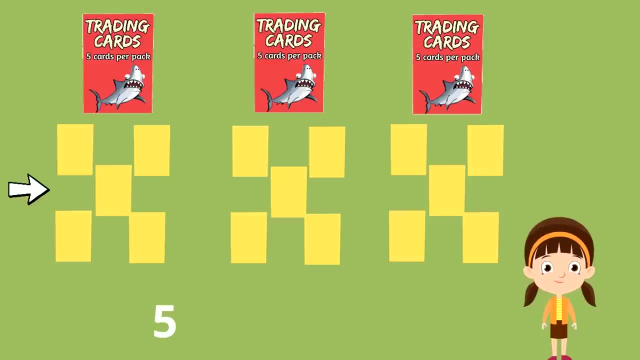 sounds like we're going to need to multiply. so each group has five. so that's the first thing. we write down the number in each group that's five. put the multiplication sign, which is the X, which means times five. times how many groups are there? one, two, three? so the second number is: 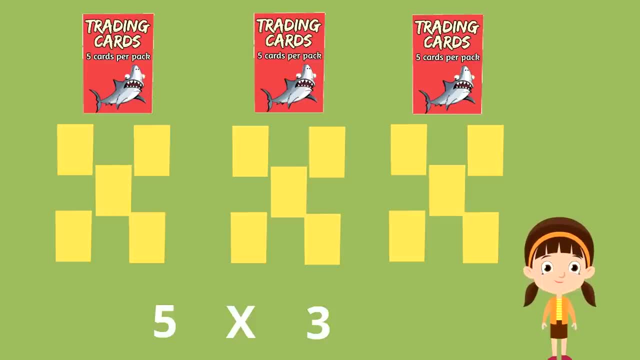 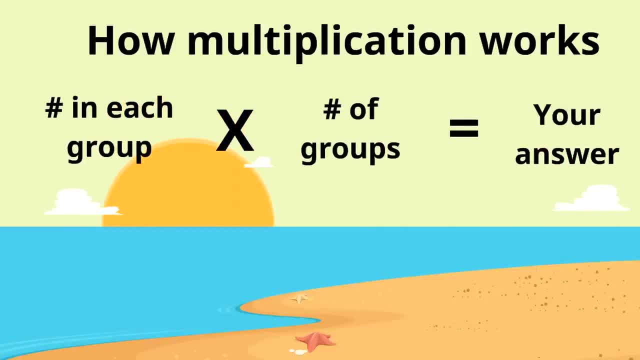 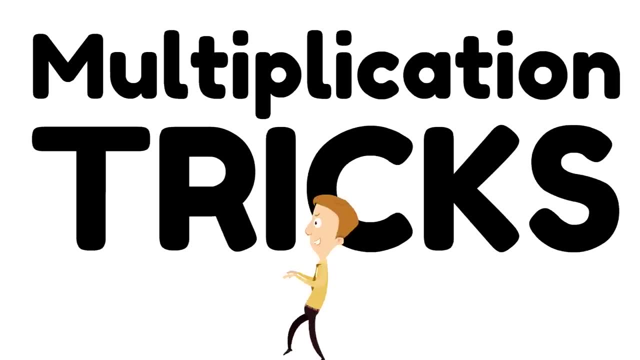 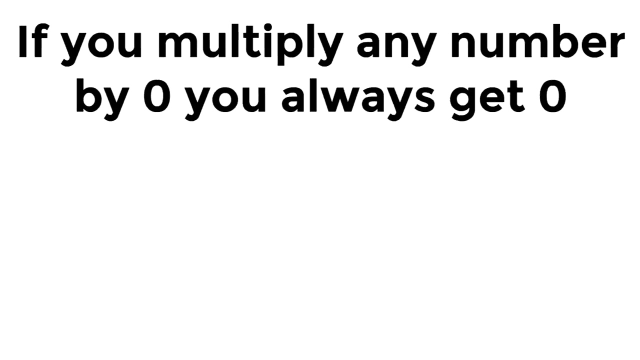 the number in each group times the number of groups and you get your answer. now here are some multiplication tricks that are gonna be really sneaky ways that you can figure out multiplication problems really, really quickly. here's the trick: if you multiply any number by zero, you always get zero, always you. 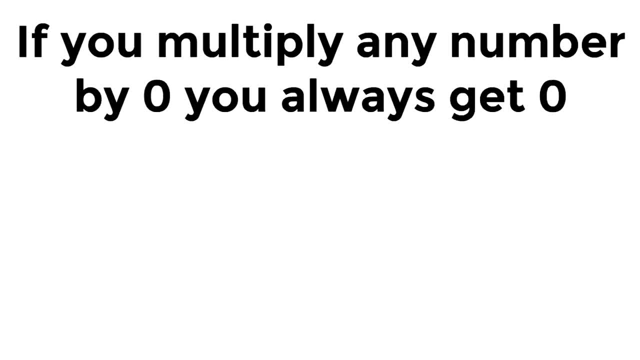 always get zero. here's an example: five times zero equals zero. when you have zero groups of five, that means you have zero. there are none. whenever you multiply any number by zero, you always get zero. 100 times zero equals zero. even if zero is the first number in the equation, you still always get zero when you multiply by any number. 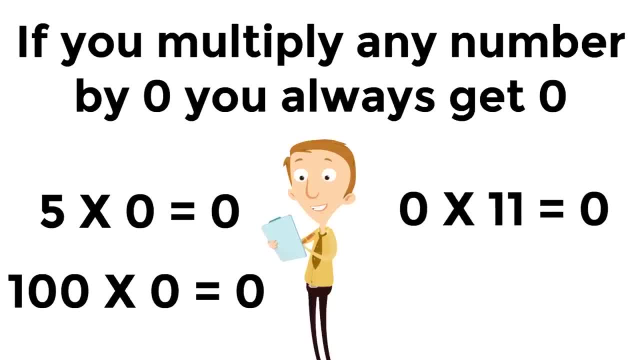 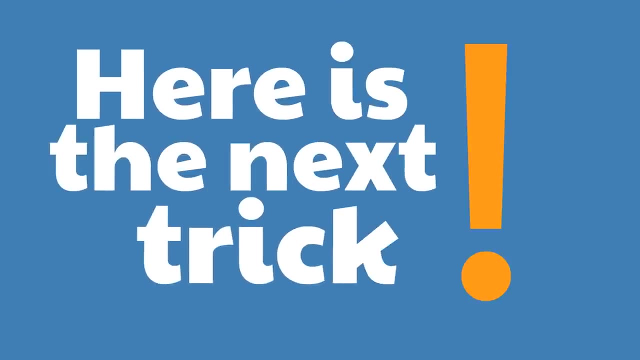 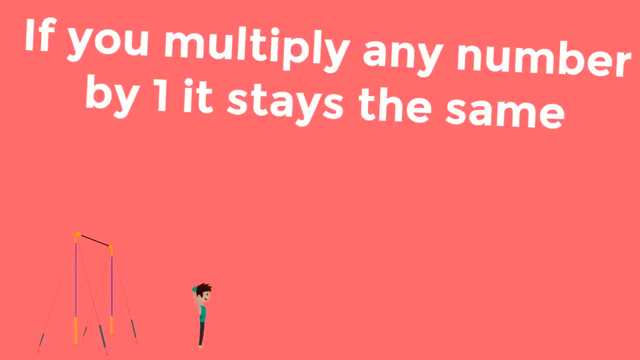 for example, zero times 11 equals zero and zero times 1000 equals zero. if you multiply any number by zero, you always get zero. oh, this has been so much fun. here is the next trick. if you multiply any number by one, it stays the same. look at these: seven times one equals seven. 100 times one equals 100. 33 times one equals 33. if you 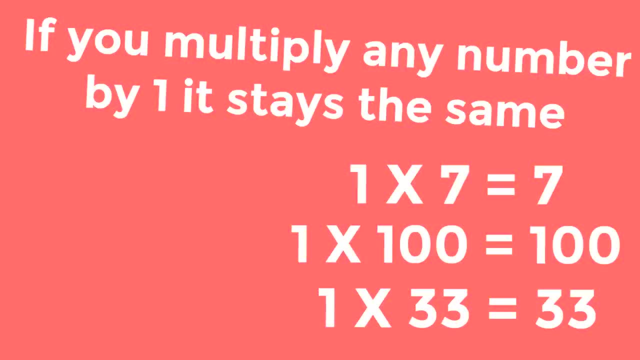 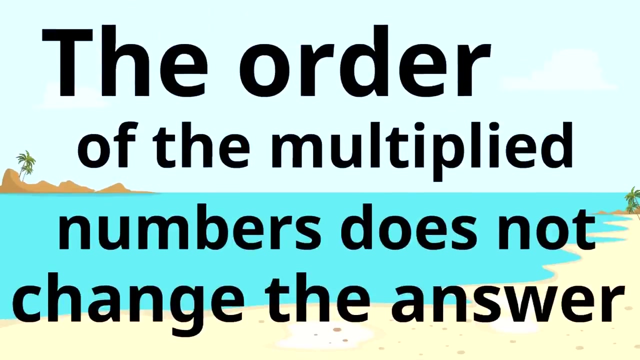 flip them, the answer stays the same: one times seven equals 7. 1 times 100 equals 100. 1 times 33 equals 33. honestly, the order of the multiplied numbers does not change the answer. if you were to flip the number of groups and the number in each group, you would. 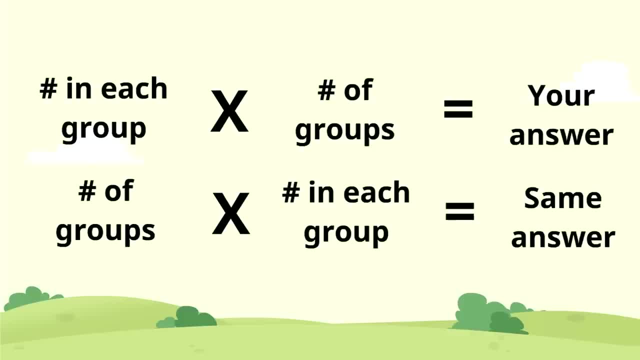 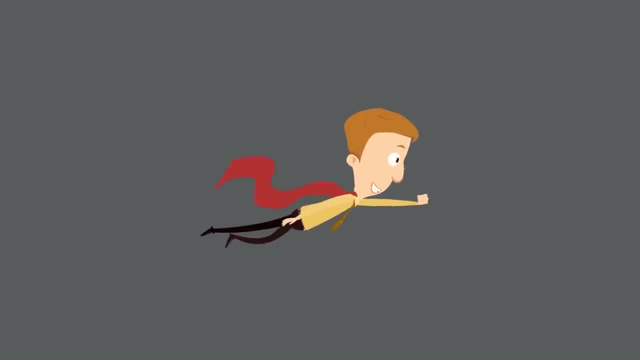 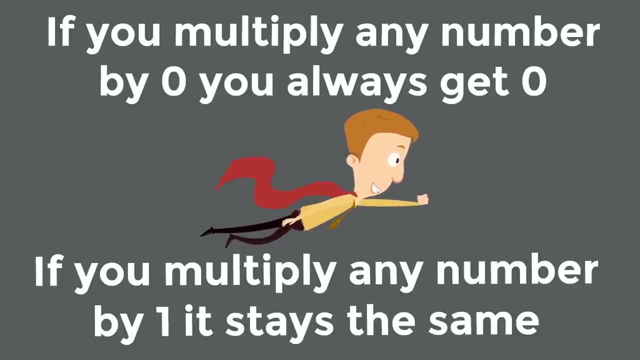 still get the same answer, though we still recommend this way, so simple. the number in each group times the number of groups to get your answer. so the two tricks have been: if you multiply any number by 0, you always get 0, and if you multiply any number by 1, it stays the same. the final multiplication trick is: 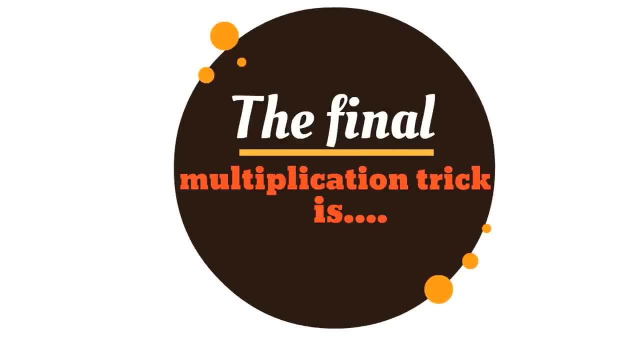 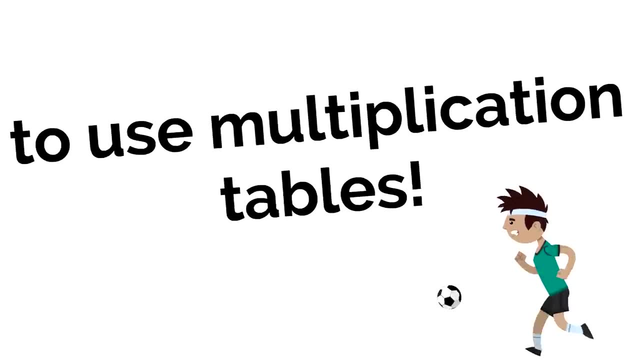 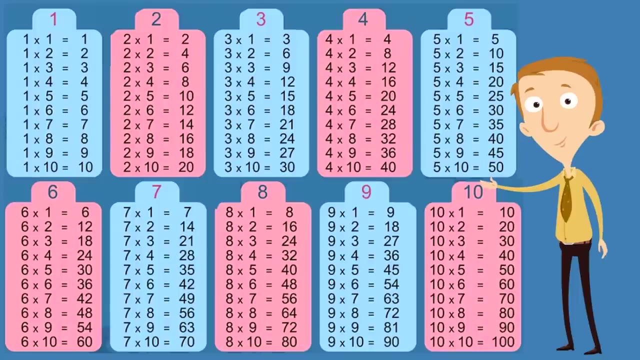 to use multiplication tables. they come in all shapes and sizes, but they are all helpful, especially as your first learning how to multiply. here are some examples of multiplication tables. there's a table for all of the numbers from 1 to 10. some kids memorize tables like these so that 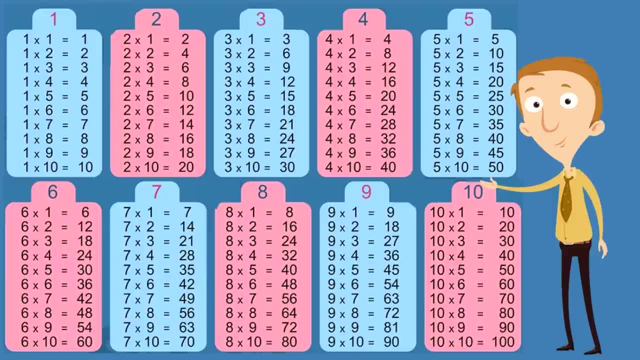 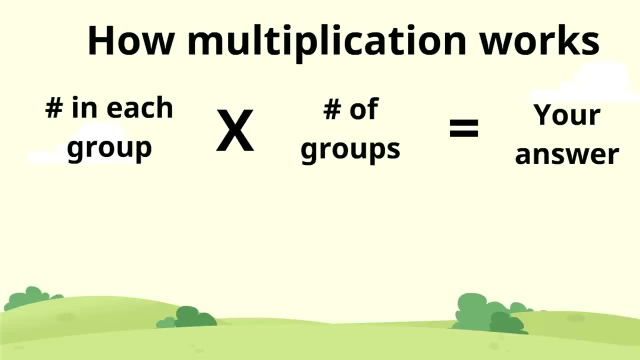 they'll know right off the bat in a moment what an answer could be for certain multiplication problems. this is how multiplication works. the number in each group times the number of groups gives us our answer. oh, this little baby's putting together a little craft. you know, it's so great I. 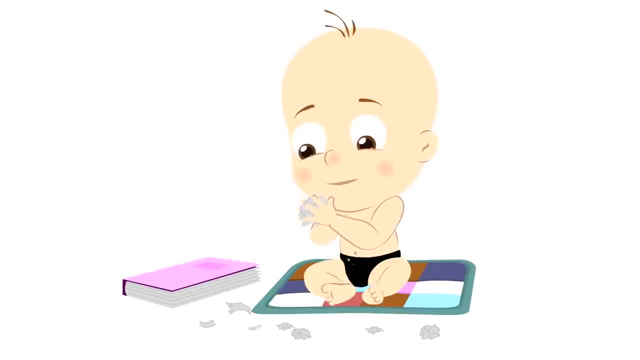 just love that. this is so good. wait a second. that that papers from that book, isn't it? ok, this is see. this is. this is not an approved arts and crafts activity right now. um, ok, we're going to have to take care of this, but first let's learn about. 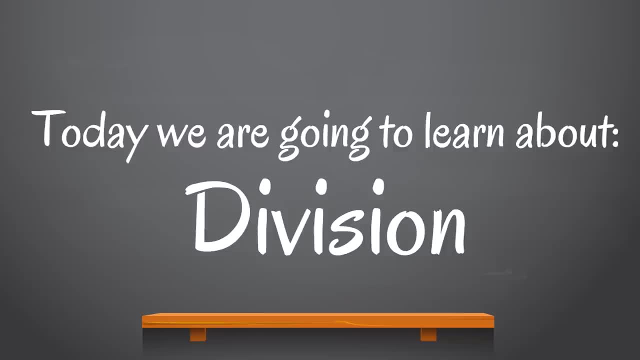 division. division is such an awesome thing to be able to do and you're going to have it all figured out. you're going to learn how to divide in this video and we're going to start off with a story. there's this kid named Ethan and Ethan. 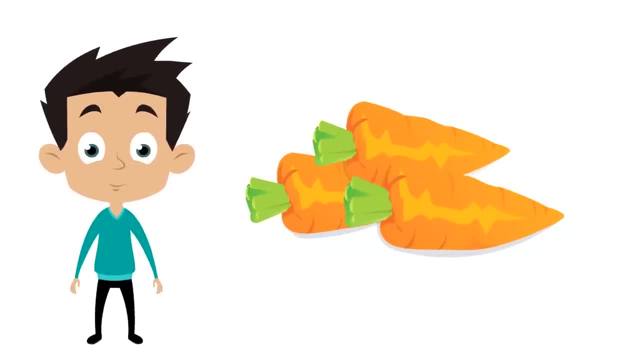 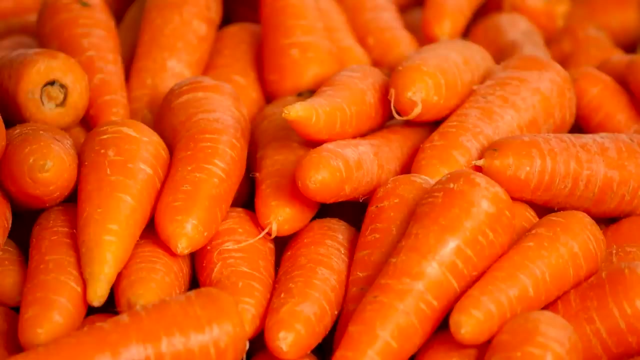 loves carrots. he loves carrots so much he loves to snack on him. he loves when he gets to eat them. they're crunchy, they're tasty. yeah, carrots are awesome. in fact, I'm literally eating a carrot right now as I'm speaking. carrots are great for your skin. carrots are great for your eyes. they're amazing. they're a. 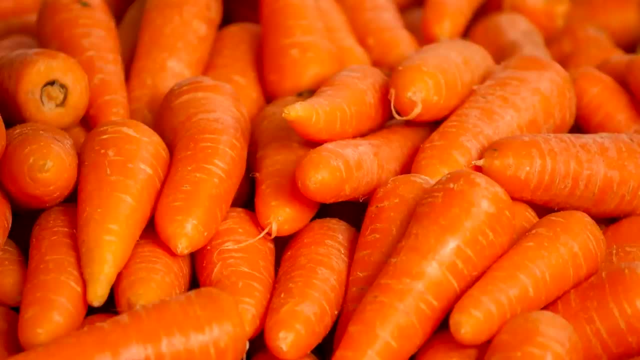 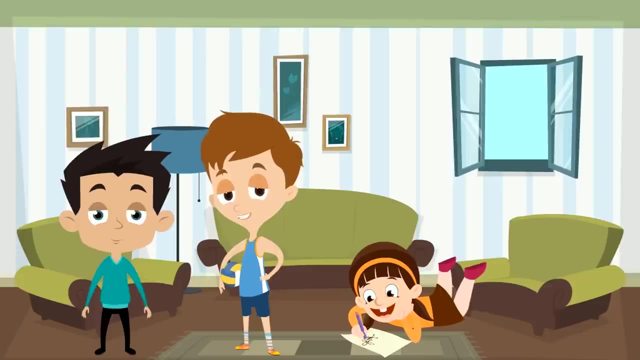 great snack and Ethan loves them. well, Ethan has two friends over, Kevin and Chloe, and they start to get hungry. of course, they all love carrots because parents are like the perfect. now in Ethan's house there are only three carrots. they're just three carrots. we are going to have to divide the three. 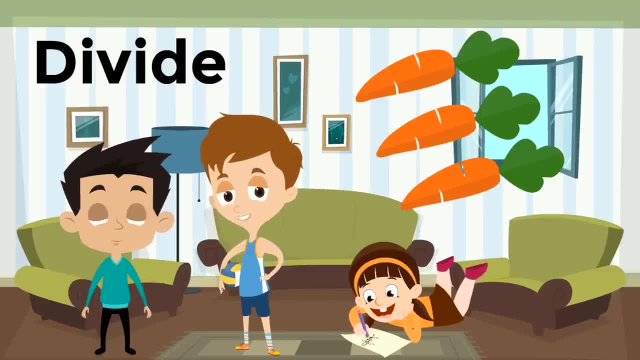 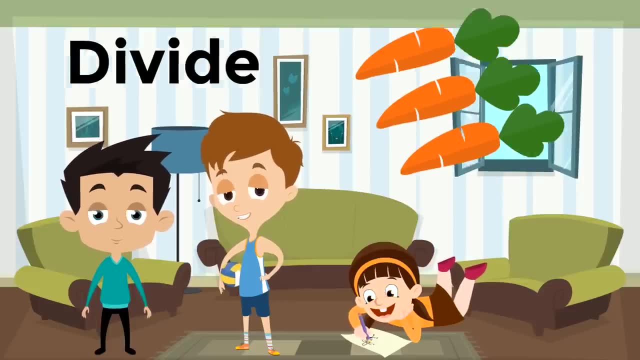 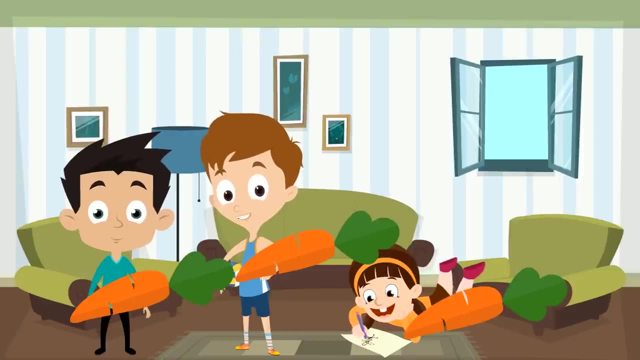 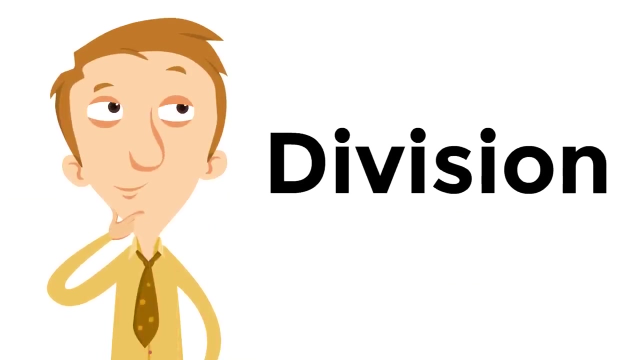 carrots amongst the three kids. so let's figure this out. how many carrots does each kid get, do you know? uh-huh, each kid gets one carrot. pretty simple, right: three carrots, three kids. each kid gets one carrot. hey, did you know? we just did division. uh-huh, we just did division. division is pretty simple, you see. 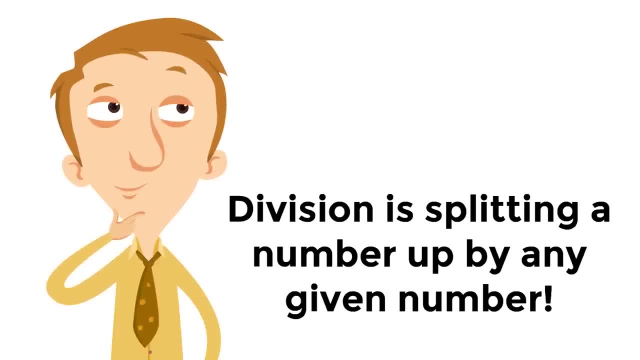 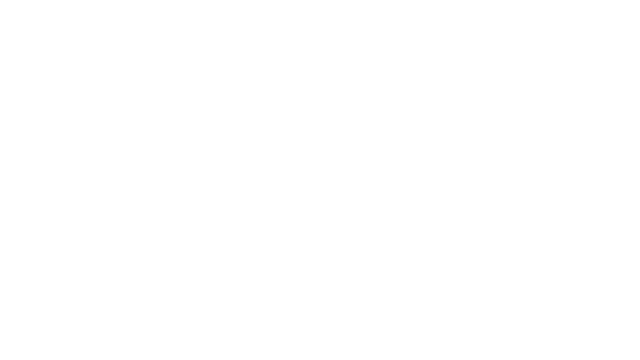 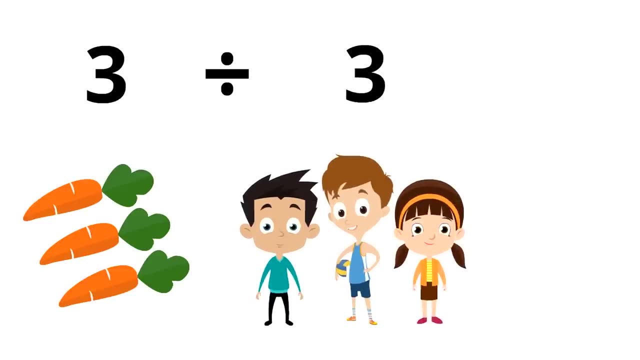 division is splitting a number up by any given number. that's it just splitting a number up. let's look at our story again. there were three carrots and we divided those three carrots and we divided them by a number, and we divided them by a number and we divided them by a number. notice, right here is the division sign. 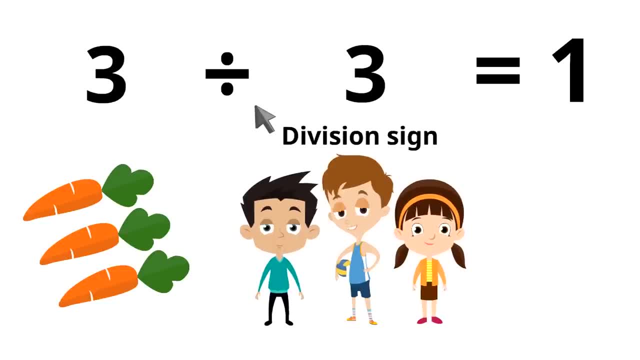 notice, right here is the division sign. this is what it looks like. when you see that sign, you could just say divided by. so this reads: three divided by three. that's the division 6 and this is the division 7 and we split in half. alright, notice right here, this is the division 6 and we divided by three. does each kid get? 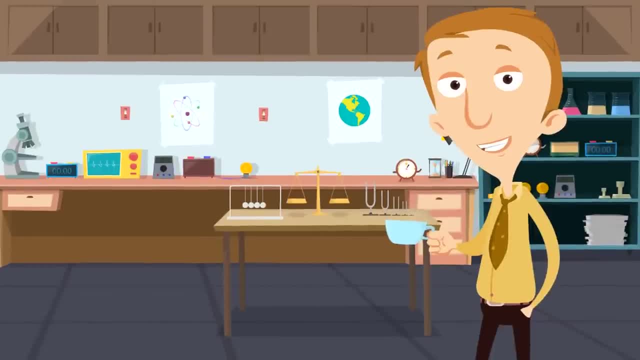 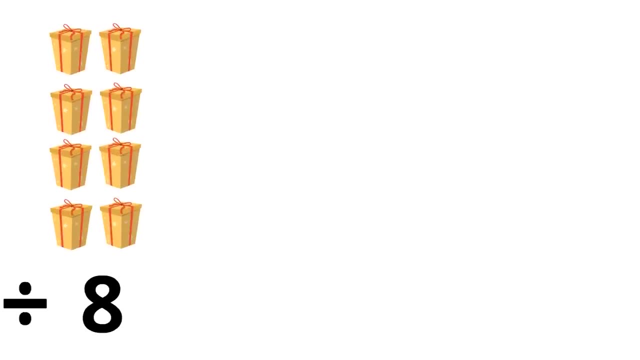 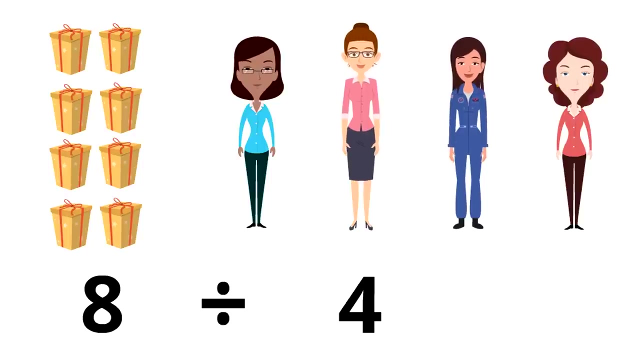 equals one. let's try another example of division. let's say there are eight presents, eight presents and there are four women, and we want each of the women to get the same amount of presents as the other women, because we want it to be fair. notice the division sign. we are going to divide or split up eight by 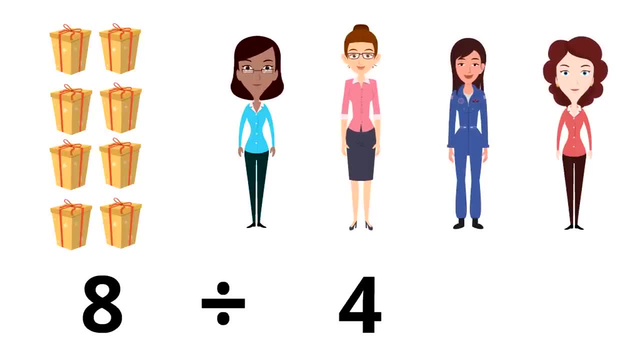 four. remember: to divide is to split up. let's split these presents up into four equal groups: one, two, three, four. all right, how many presents does each woman get? uh-huh two. each woman gets two presents. isn't that cool. division is so much fun and it's so easy. 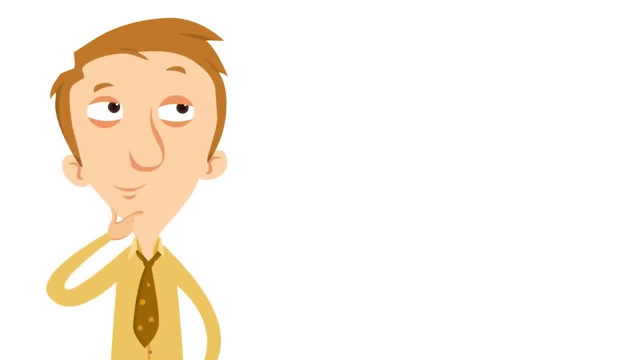 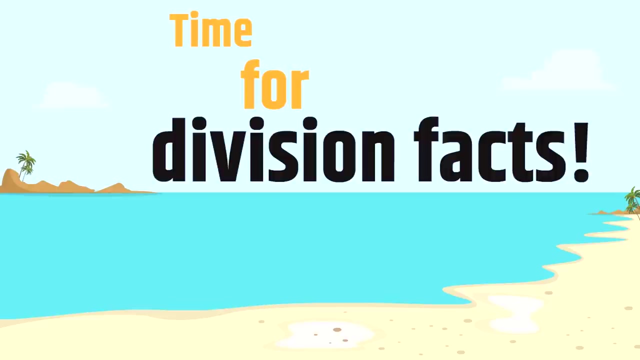 you remember, division is splitting a number up by any given number. that's it all. right. now it's time for division facts. we're going to learn some pretty interesting facts about division and you're gonna be like what? oh my goodness, like secrets, this is super cool, okay, so just look around. all right, make sure. 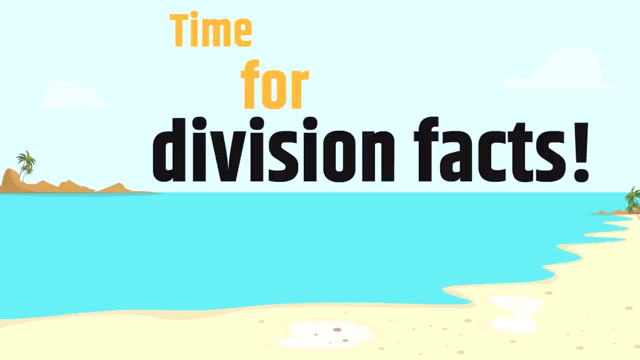 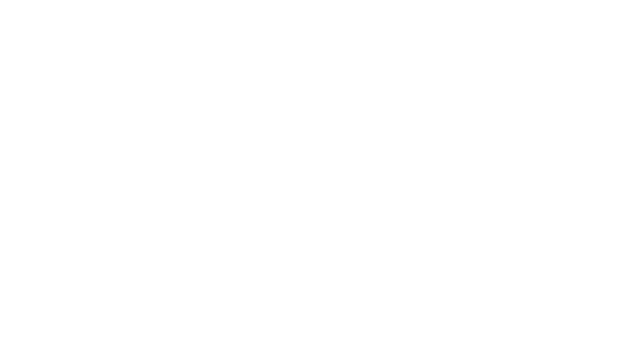 who's clear. all right, it's time for division facts. the first fact is this: you can never divide by zero. it's true, you can never divide by zero. even if you're a rule breaker and you're like: I'm gonna do whatever I want, you still can never divide by zero. in fact, 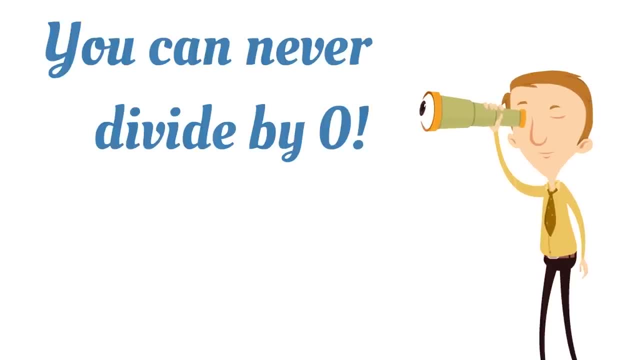 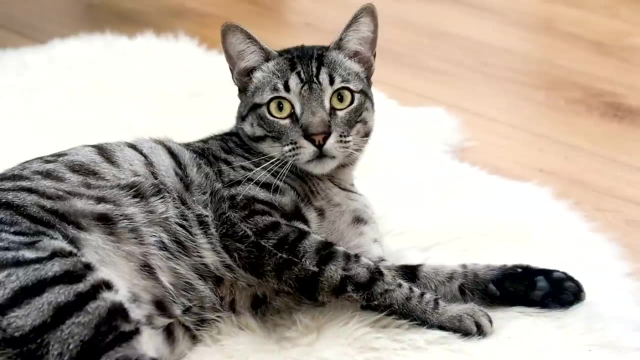 if a teacher ever gives you a test and you see a problem where you have to divide a number by zero, just right on the test- undefined, because that's exactly what that answer would: be undefined, it's impossible. kind of like mr whiskers math skills. does mr whiskers do math in his head all day long? who knows his math? 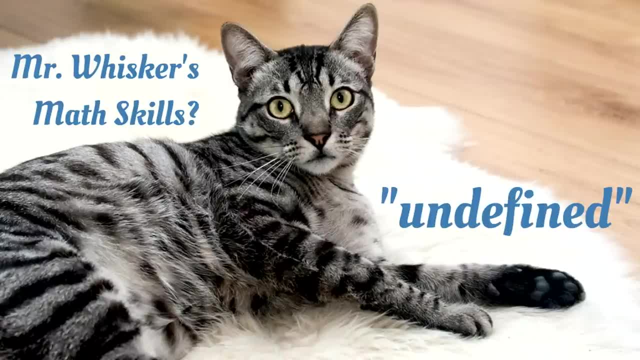 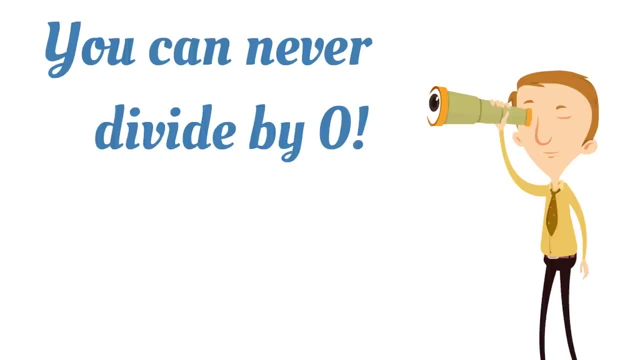 skills are undefined. we just don't know. it's impossible to know. you know, mr whiskers might know how to do division, who knows? undefined. you can't divide by zero. you can never divide by zero. if you ever see any division problem dividing by zero, just write: undefined, it's impossible. it's impossible, so just write. 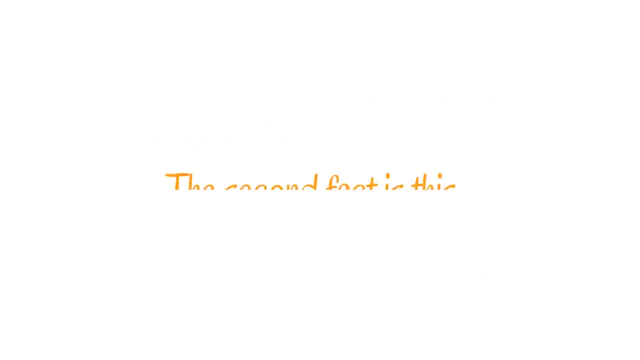 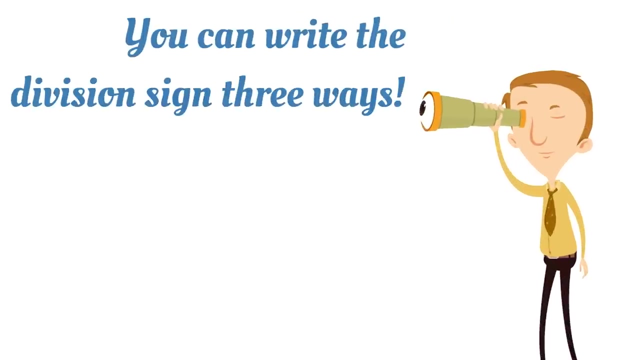 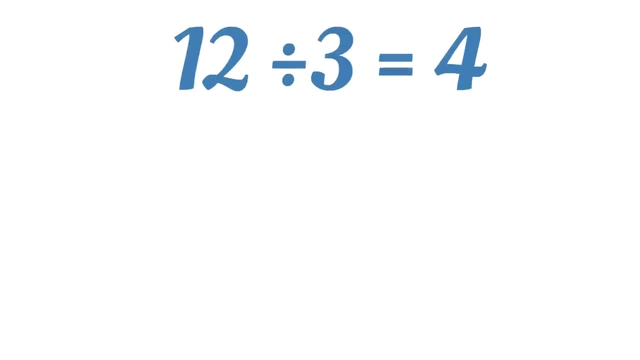 undefined. the second fact is this: you can write the division sign three ways, uh-huh, not just with that traditional division sign. you can write it like the division sign, or you can write a division problem with the slash or with a horizontal line, for example. look at this: 12 divided by 3 equals 4. that's the original division sign, the. 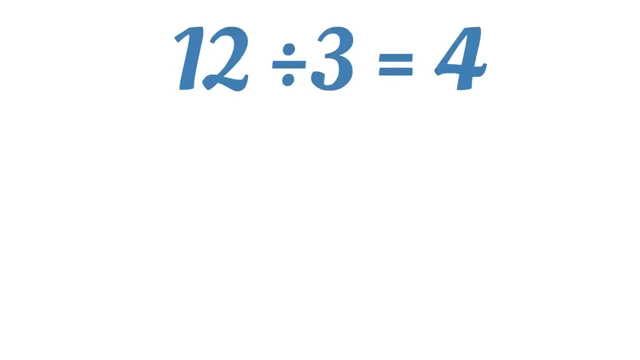 one that you might see more regularly. but here is the same equation written in a different way: 12 divided by 3 equals 4. it's still a division sign, but it's a slash. it means the same thing as the original division sign. remember, the division sign can also be a horizontal line: 12 divided by 3 equals. 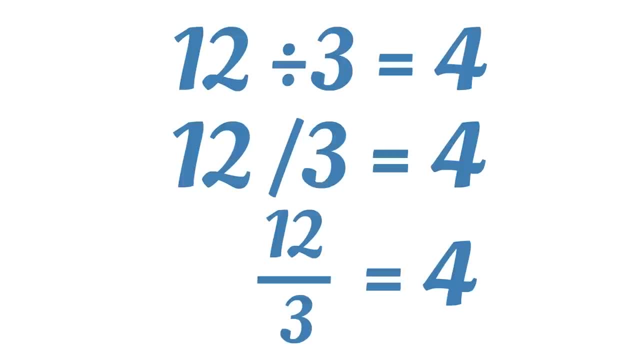 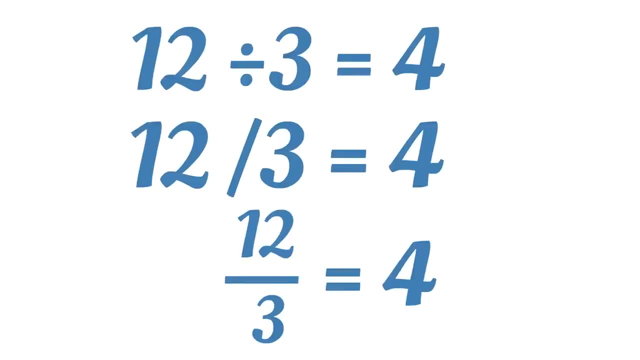 4. that looks like a fraction, doesn't it? the line in a fraction means divided by zero. these are the three ways that you can write the division sign. pretty interesting. all right, the final fact is this: this is so awesome: you can select the number of groups and the number in each. 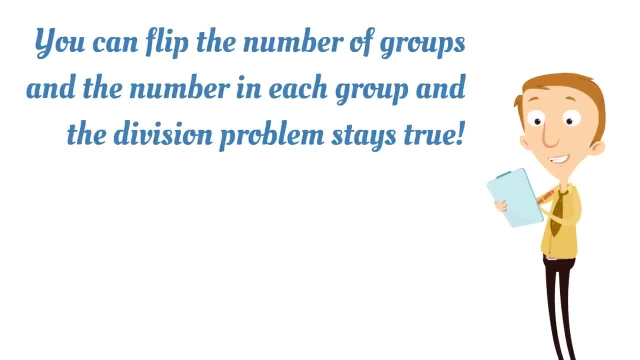 group and the division problem stays true. for example, 10 divided by 2: two equals five. and you can flip the two and the five and it stays true. that means 10 divided by 5 equals 2.. isn't that interesting. 10 divided by 2 equals 5. 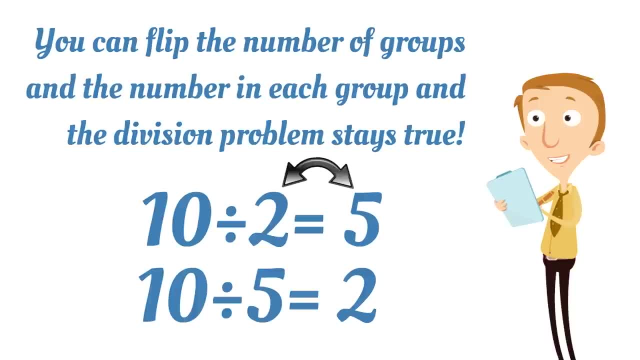 and 10 divided by 5 equals 2.. you can flip the number of groups and the number in each group and it still stays true. or look at this: 18 divided by 6 equals 3.. remember, we can flip the number of groups and the number in each group and it still stays. 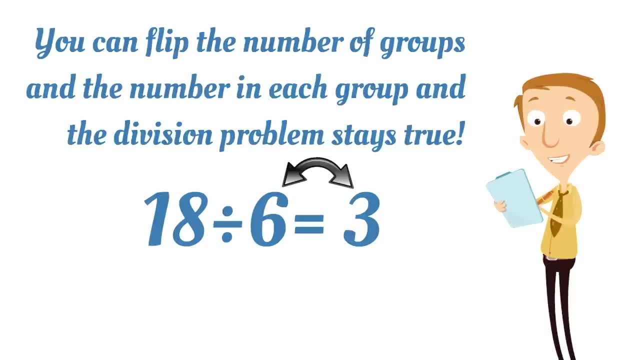 true, so we could switch the 6 and the 3 and it stays true. so 18 divided by 3 equals 6.. the 6 and the 3 can be flipped, so 18 divided by 6 equals 3 and 18 divided by 2 equals 3.. 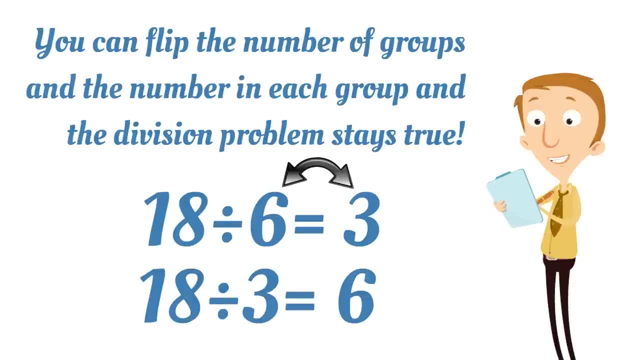 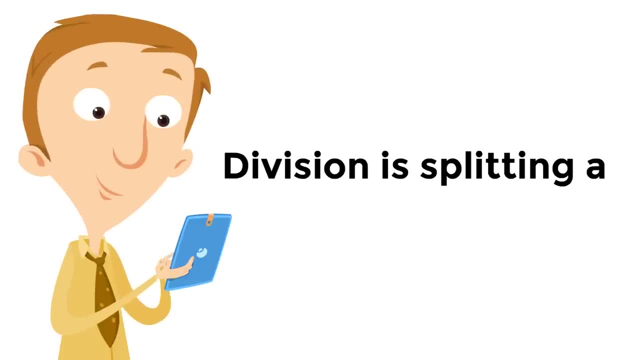 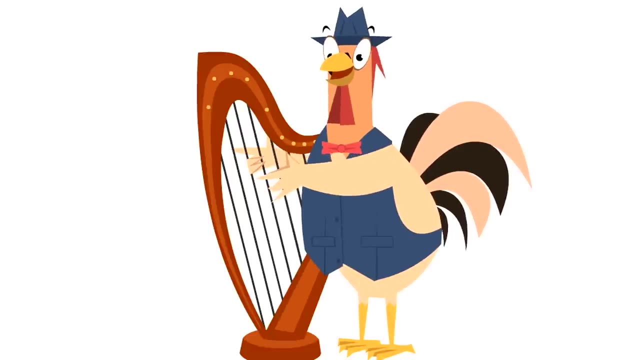 to buy three equals six. pretty nifty. those were some cool facts. you know, division is a great time. division is splitting a number up by any given number. it's a lot of fun and we hope you learned a whole lot in this video. here's our friend fred. we heard that he just took up the harp. he just 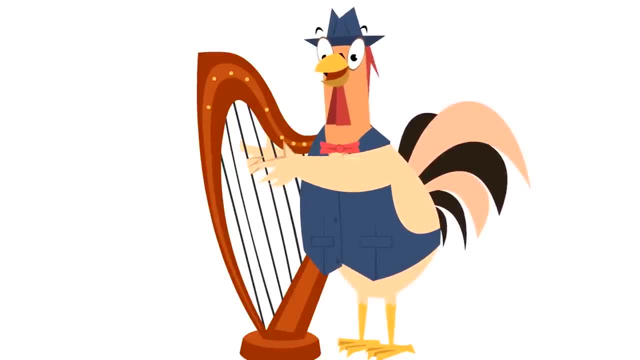 started playing the harp, fred, we can't. we can't hear. we're having audio problems with fred right now. fred, you look so happy playing, we, we can't hear you. okay, you've got, you got to wear your mic or something. we can't hear the music he doesn't even know, he doesn't even, isn't that? 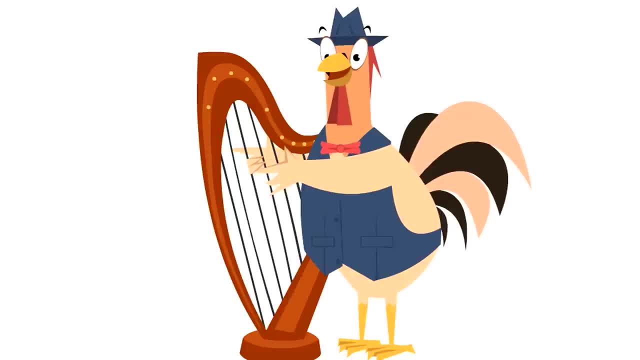 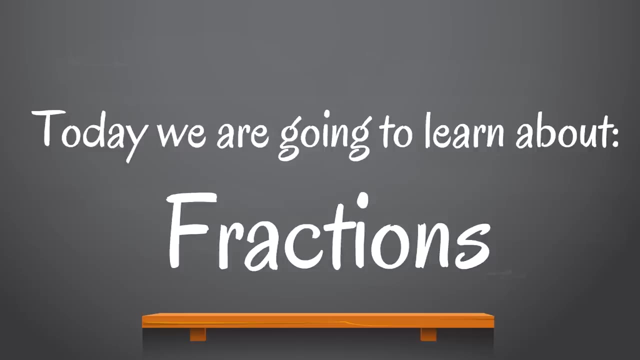 nice. you know, fred is just plucking away. he's having a good time. you know, kind of like we're having a good time right now with these learning videos and next we are going to learn about fractions. fractions are so awesome and so much fun. many of you think so too. 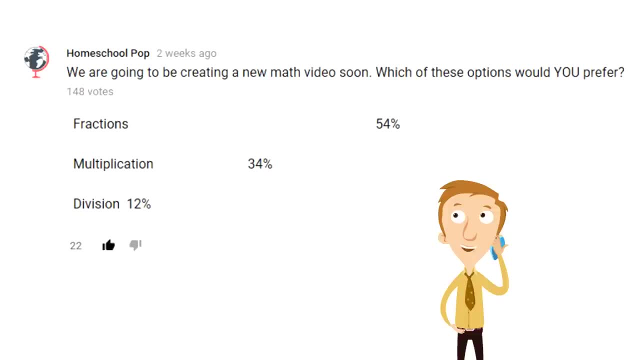 okay, couple of weeks ago, we set up a poll on our channel and many of you voted for fractions as our next math video. that's really awesome. thanks everyone for voting and don't worry, we'll make the other two videos too, later on. but this is all about fractions, all right? well, let's start here. 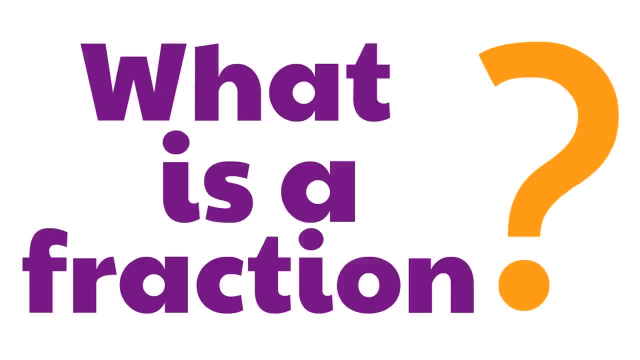 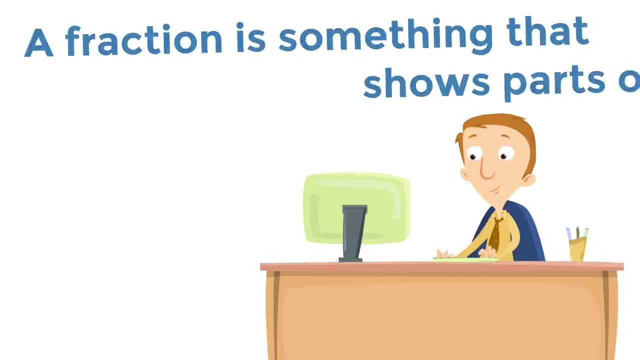 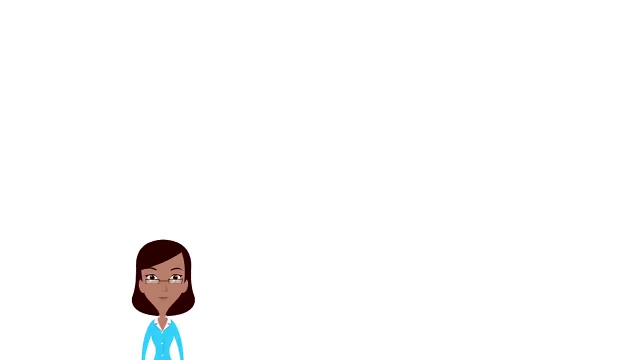 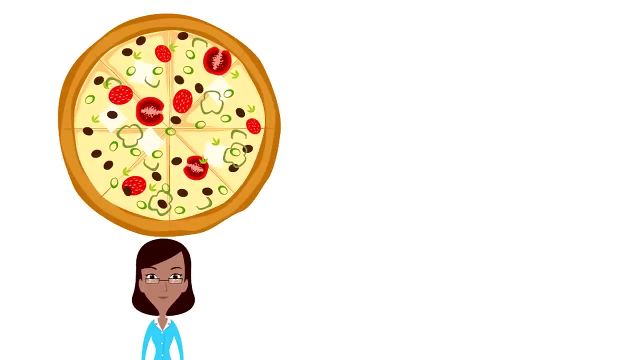 what is a fraction? when we say the word fraction, what do we mean? what is a fraction? well, a fraction is something that shows parts of a whole. let's say there's this lady named cindy. cindy has a pizza, which is great. she loves pizza, so yummy pizza. 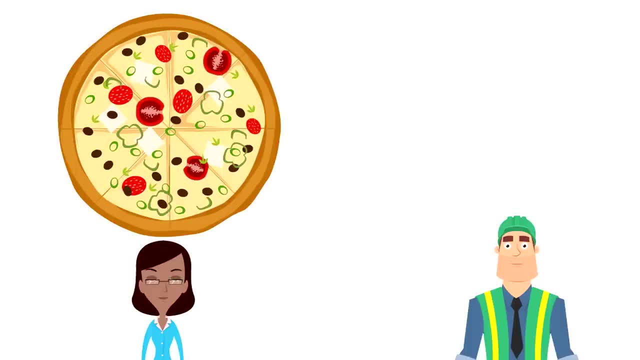 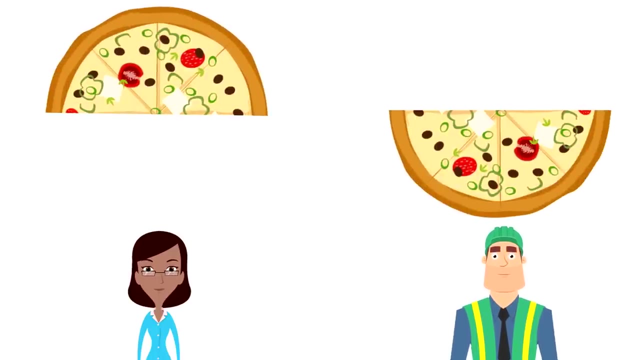 but then her friend chomsky arrives. you remember chomsky. chomsky likes pizza too, and he's a little bit hungry. so maybe cindy isn't gonna eat the whole pizza now. maybe they're gonna split it. what do you think? so they split the pizza in half. each of them get. 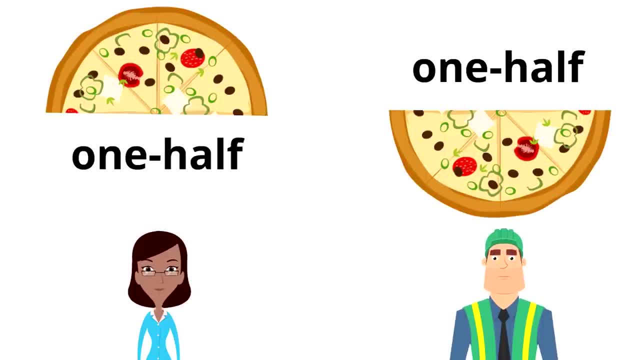 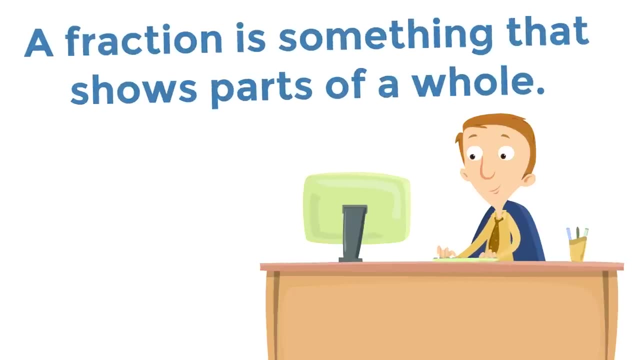 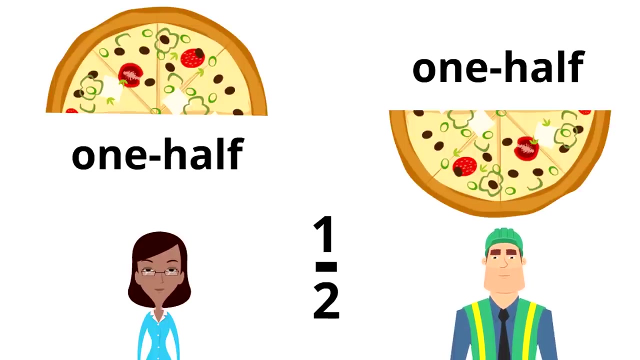 one half of the pizza. that neat. then everyone has pizza. each of them have one half of the pizza. they split it right down the middle. now remember, a fraction is something that shows parts of a whole. so here is what the fraction looks like: a one, a line and the two. that is the fraction: one half. 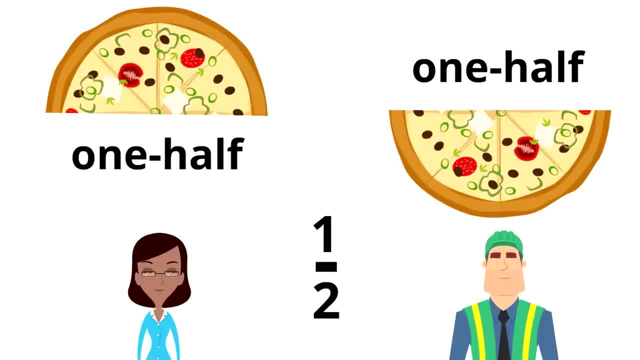 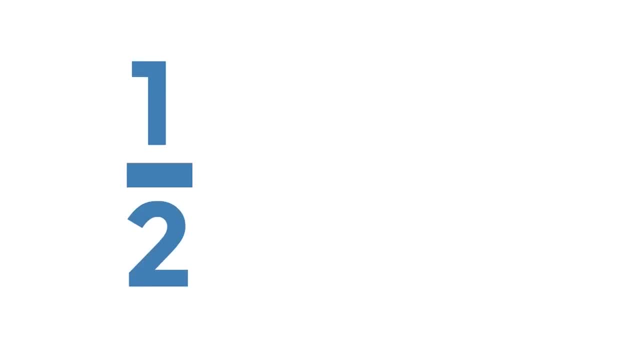 each of them, cindy and chomsky, get one half of the pizza. so this is one half. it's a very important fraction because we use it all the time. now you might be wondering what do the numbers mean and how does it show one half? well, the bottom number shows the total number of parts. 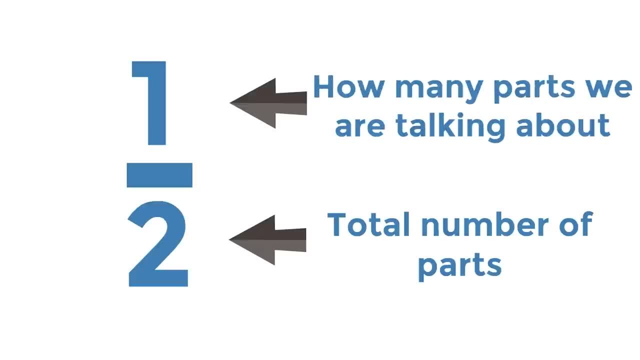 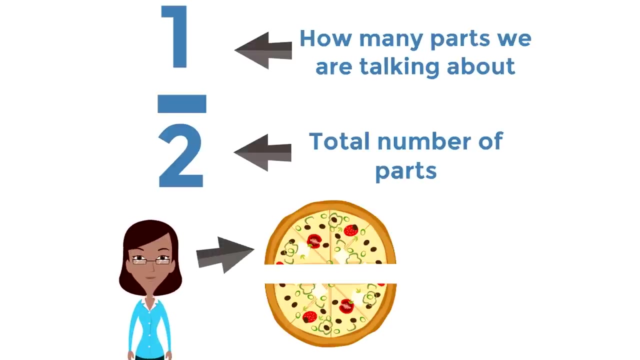 the top number shows how many parts we are talking about- pretty simple. let's go back to our example. there are a total of two parts to the pizza, so there's a two on the bottom and cindy just gets one part. that's the part we're talking about. 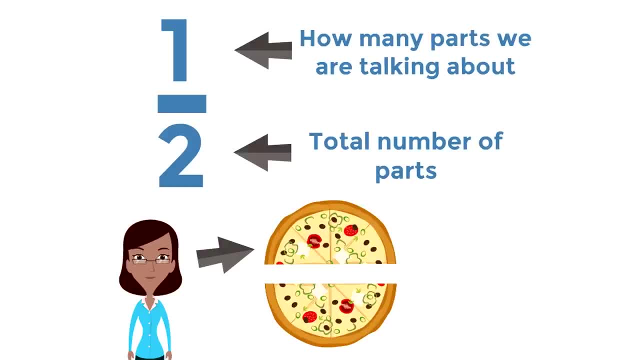 so cindy gets just one half of the pizza. she doesn't get the whole thing, she gets just one part. she gets one half. the bottom number of a fraction is called the denominator. the denominator is the total number of parts. the top number is called the numerator. the numerator tells us how many parts we are talking. 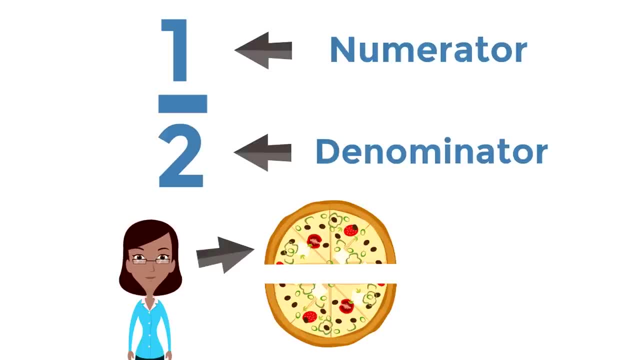 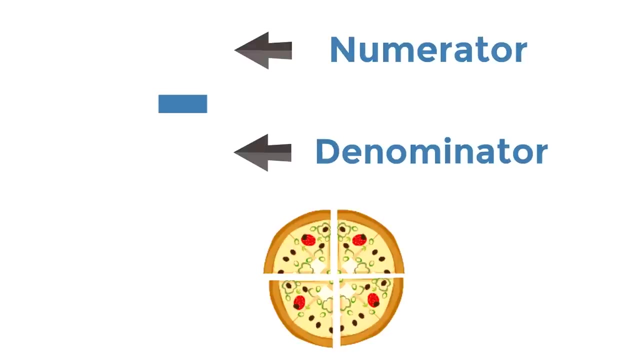 about. in this case, cindy is having one part of the pizza. the other part, of course, is going to chomsky. let's try this. let's say there's another pizza and this pizza has four parts. the number four is the denominator, because there are four pieces of pizza, four parts. 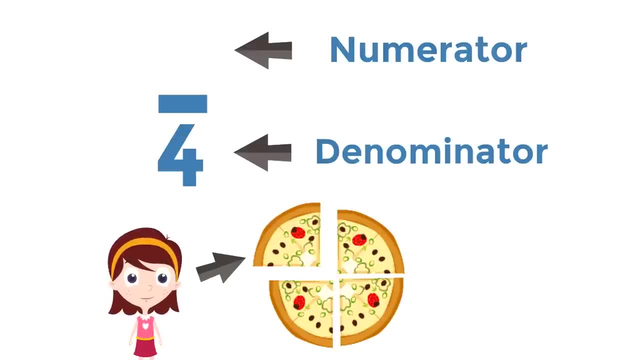 are the upper part, so we're talking about one half of the pizza and cover. the other half of. that is for Arrowhead America, for Yahoo, butterナ, multiple parts and lastly, cindy gets the answer for the. the pizza is doesn't need to be four parts to get to the bottom, because it also does that. 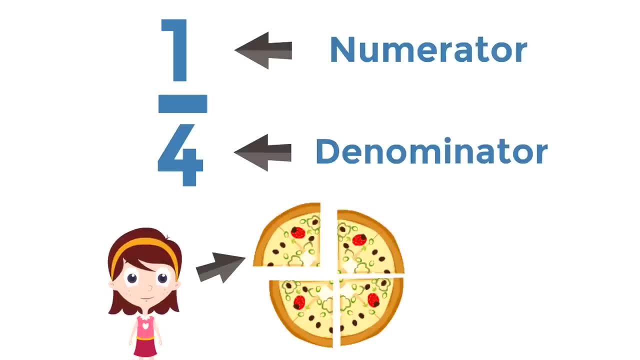 ja mentioned earlier in the rubric that kelly shows up and wants to have one part of the pizza, one piece of the pizza, The numerator or the top number of the fraction is 1, because kelly is having one part or one piece of the pizza. 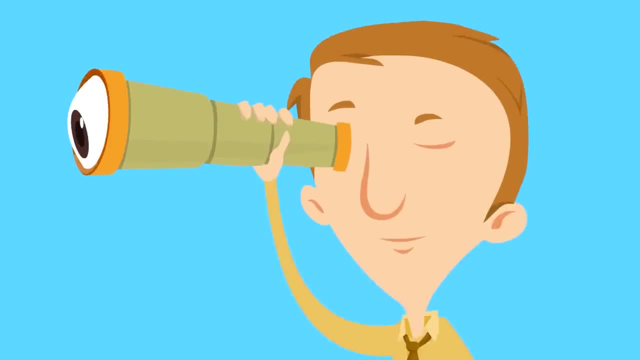 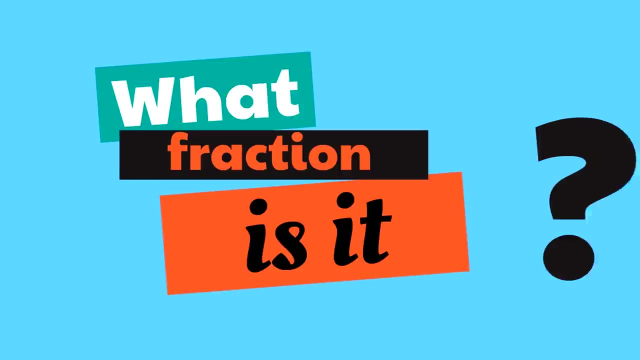 kelly is having 1 1⁄4 of the pizza. pretty simple, pretty fun fractions are awesome. 1 1⁄4 of the f? els a pretty simple, pretty fun fractions are awesome. now we're gonna need your help. help us figure out what fraction is it. huh what? 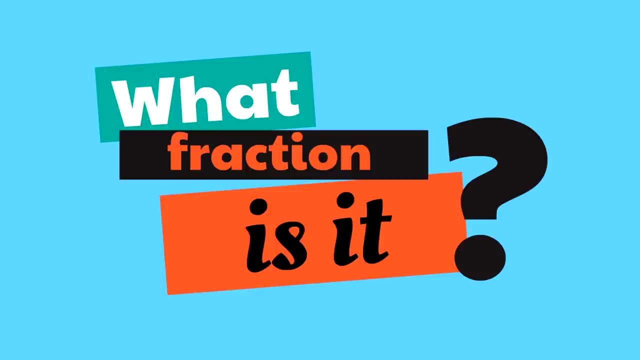 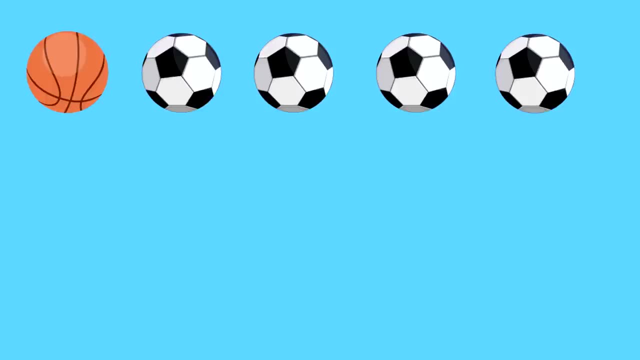 fraction, is it? wow, we're gonna have a great time. let's say we have a group of five sports balls. one is a basketball, the other four are soccer balls. let's figure out what fraction of the balls are basketballs, what fraction of the balls are basketballs. so we know a fraction has a line in the middle and 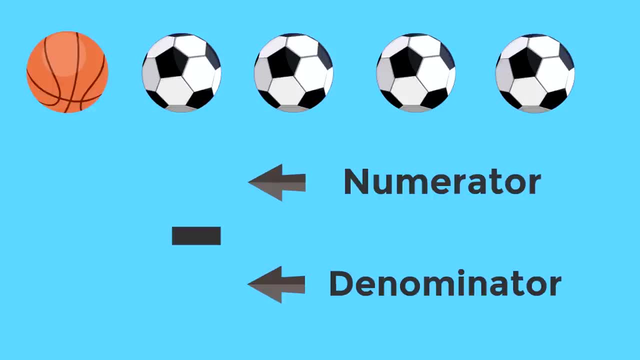 the top number is the numerator and the bottom number is the denominator. the denominator shows us the total number of parts or units. how many sports balls are there? yeah, five, five is the denominator. good job. now remember, we're asking for the fraction of sports balls that are basketballs. so how many basketballs are? 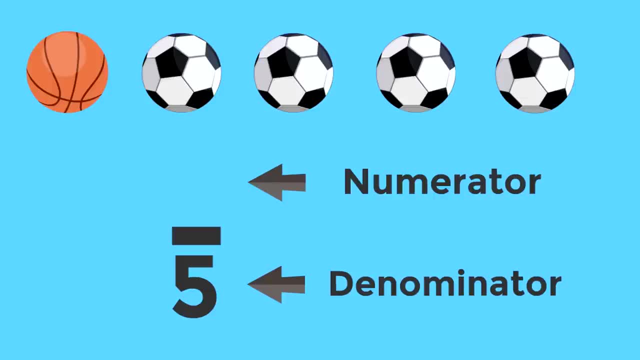 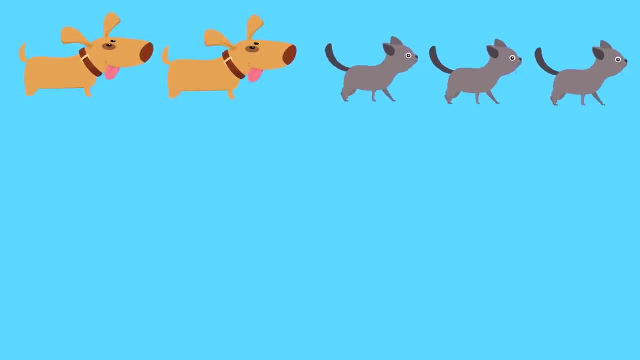 there. yeah, just one. the number one is the numerator. so, one-fifth, the sports balls are basketballs. one-fifth: great job, let's try this final example. let's say there are five pets, five pets: two of them are dogs and three of them are cats. 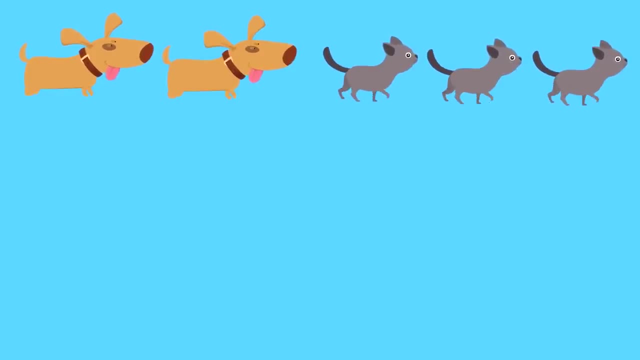 what fraction of the pets are cats? huh, that's a good question: what fraction of the pets are cats, remember? here's what a fraction looks like. it's got a line in the middle with the top number being the numerator and the bottom number is the denominator. so the total number of pets is five. what number is the denominator? 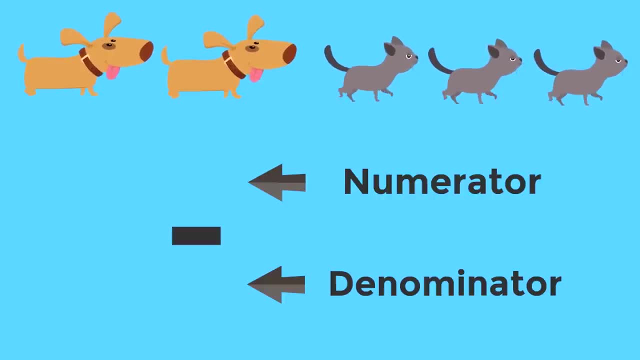 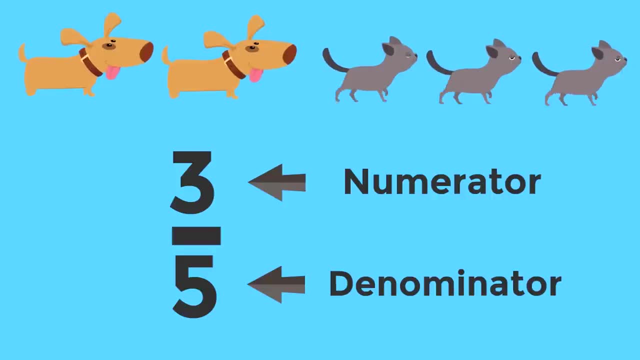 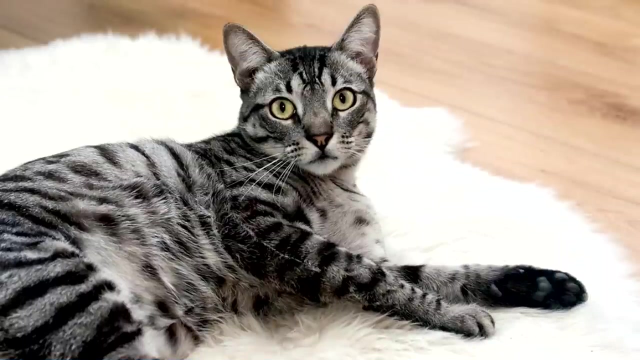 yeah, three, three is the numerator. three fifths of the pets are cats. wow, that was yeah, three. three is the denominator. three fifths of the pets are cats. wow, that was so cool. but none of those so cool. but none of those cats are special, to put you, mr whiskers, not even. 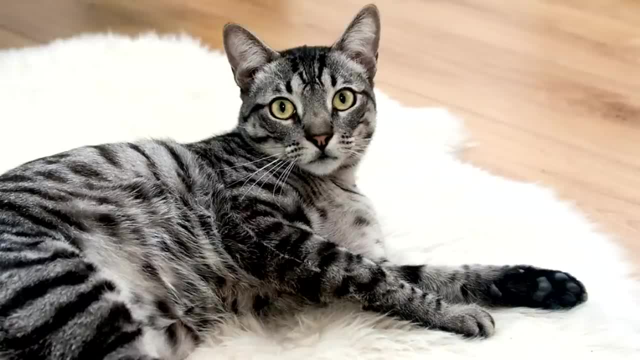 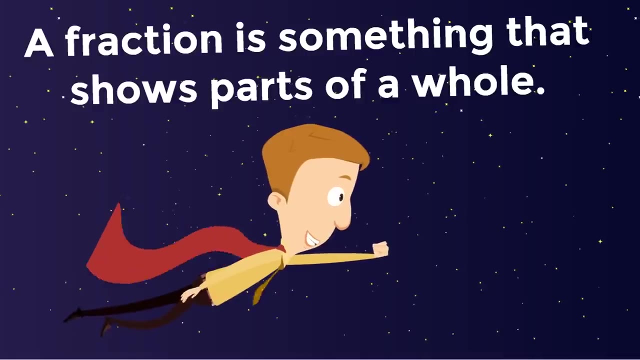 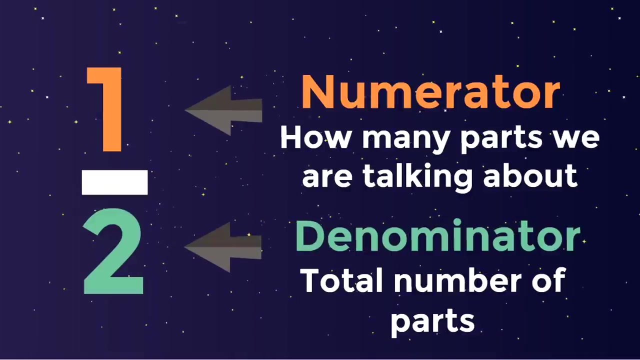 cats are special, to put you, mr whiskers, not even a fraction of my heart belongs. a fraction is something that shows parts of a whole. a fraction is something that shows parts of a whole. the top number of a fraction is the numerator. a is the numerator how many parts we are talking about? and the bottom number of a fraction is the. 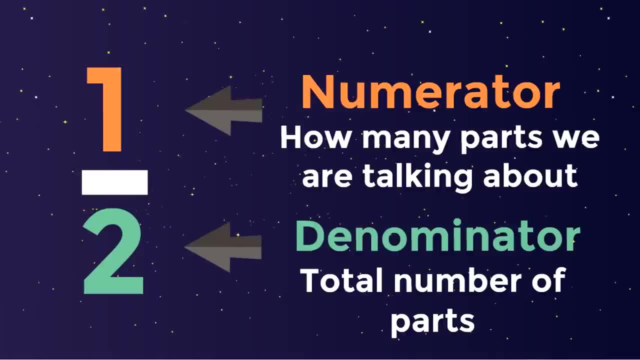 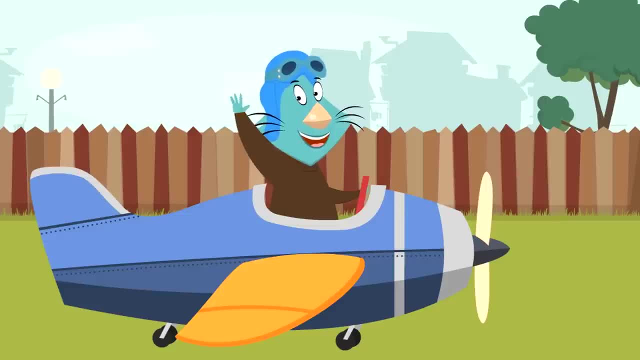 denominator: the total number of parts. Hey, Petey, I know, I know I heard about your plane. you know it's a cool plane, you know, and and it's, it's neat- I don't know if it flies or you- you look. 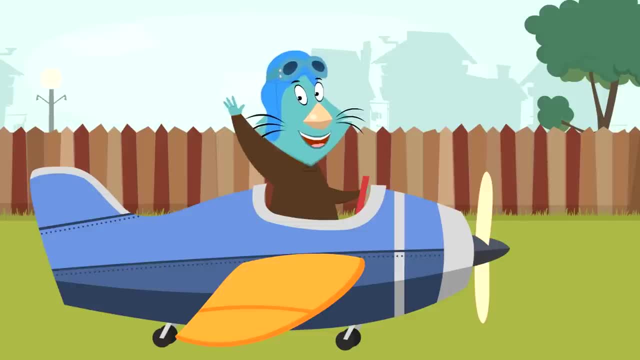 pretty confident that it's gonna fly, which is cool. yeah, I, I see you, hello, hello. yeah, thanks for waving, thanks for saying hello. you know, we're actually in the middle of learning. we're, we're in the 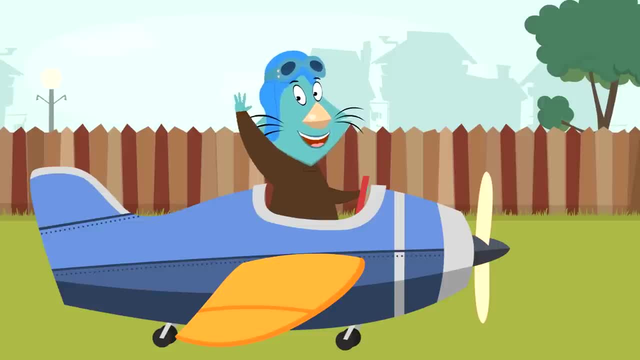 middle of learning a lot of new cool things right now, so I actually do have to go. hi, you're still waving. okay, we're gonna go, because now we need to learn about perimeter. All right, let's show you how. 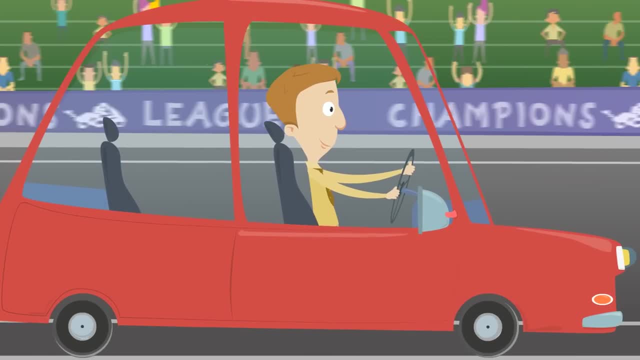 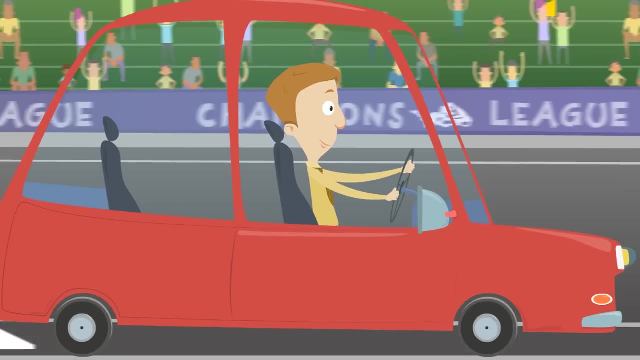 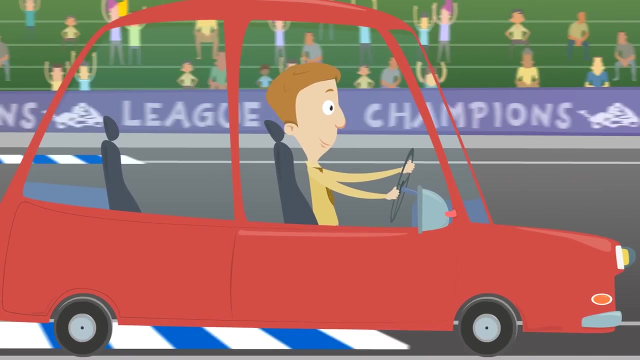 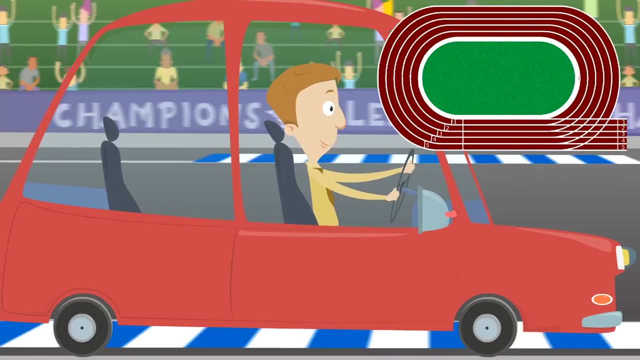 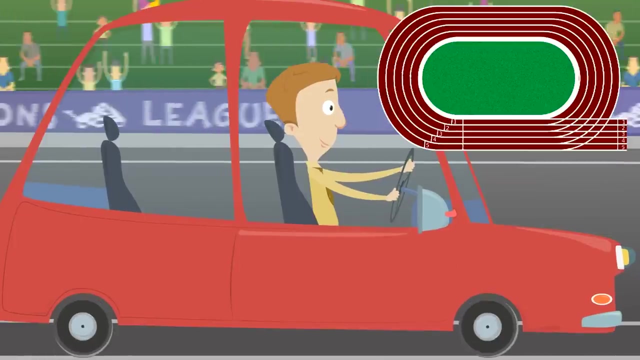 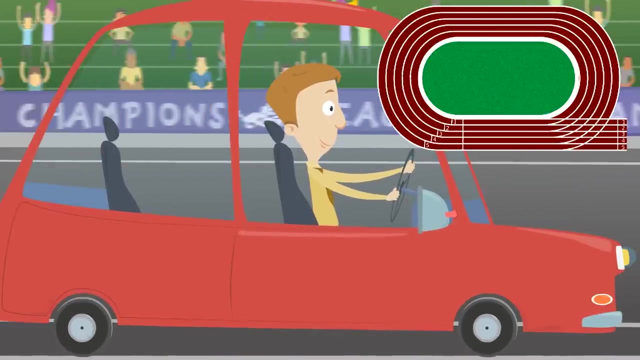 fun this is. imagine I'm a race car driver, right, and don't make fun of my car. okay, this is. this is a perfectly good car to do a race car. Race it, right, it's very fast, it's it's got the bells, it's got the whistles, it's a great race car. okay, stop laughing at it. okay now imagine this is the race car course that I'm driving on, right, it's going around an oval, it's going around a shape. if I was wondering how far is it around the track, what's the distance around the shape, then I would need to know the perimeter, the 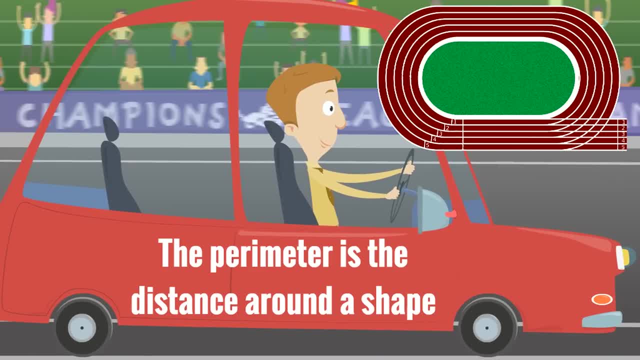 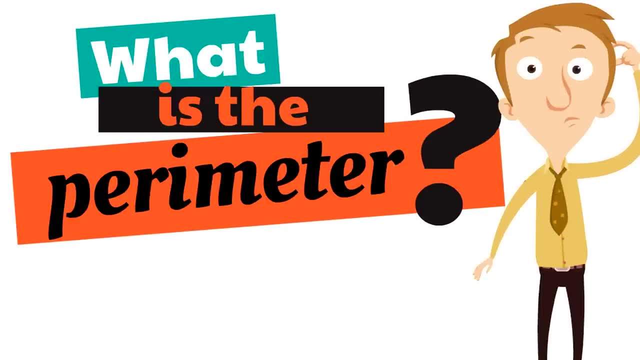 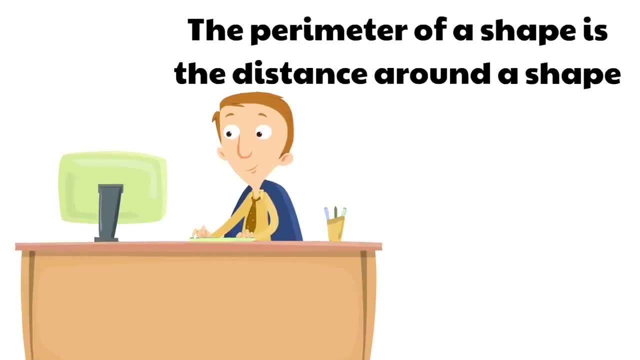 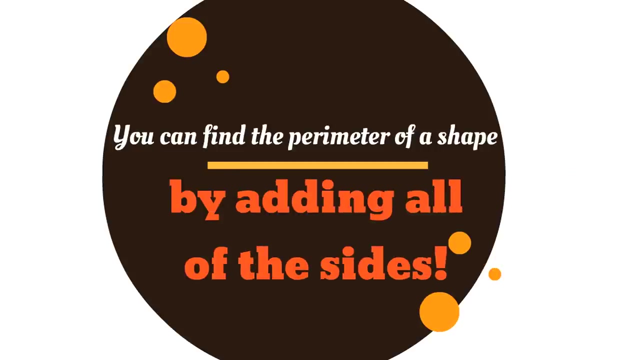 perimeter is the distance around a shape. wait, wait, wait. what is the perimeter? the perimeter of a shape is the distance around a shape, and it's easy to find. you can find the perimeter of a shape by adding all of the sides. that will tell you what the distance around the shape is. 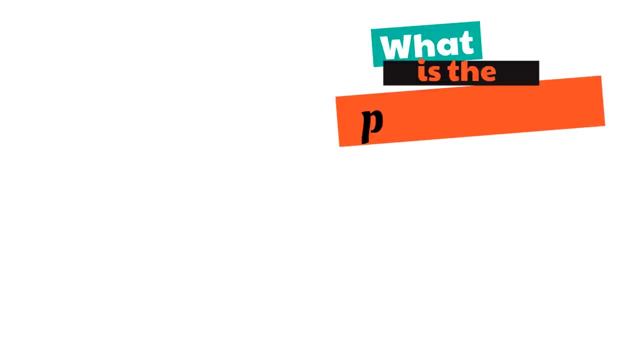 great, now let's practice finding the perimeter. look at this triangle. what is the perimeter of this triangle? okay, first we need to know how long all of the sides are. then we can figure out the perimeter. with this triangle, all three sides are the same length, so how long are they? let's pretend we measured it. 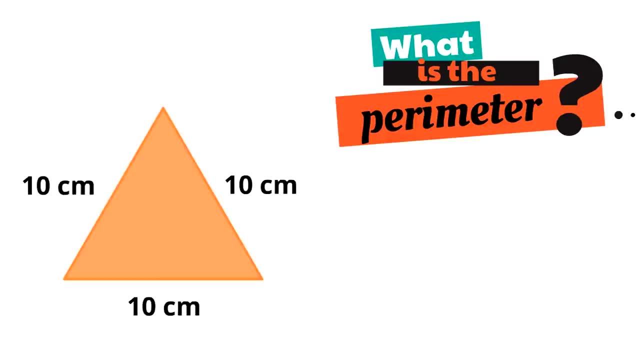 and each side is 10 centimeters. now remember: to find the perimeter of a shape, we need to know the distance around the whole shape. so we just add the sides together. what's 10 plus 10 plus 10, that's three tens. what does that equal? yeah, 30,. awesome. the perimeter of this triangle is 30 centimeters. 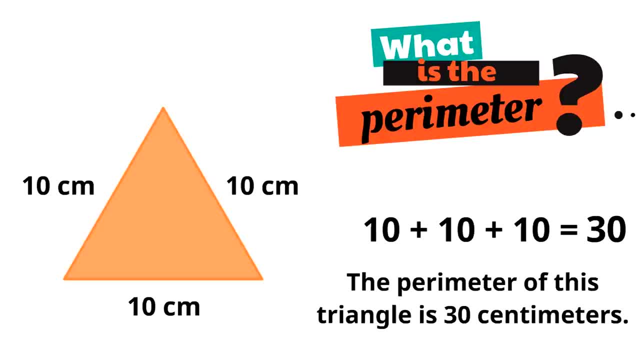 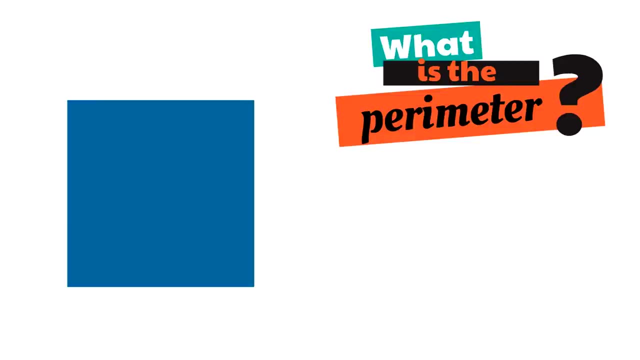 remember: cm is an abbreviation for centimeters. 30 centimeters is the perimeter of this triangle. okay, let's try this one. what is the perimeter of this square? first, we need to know how long all the sides of the square are. then we can figure out the perimeter of the square. 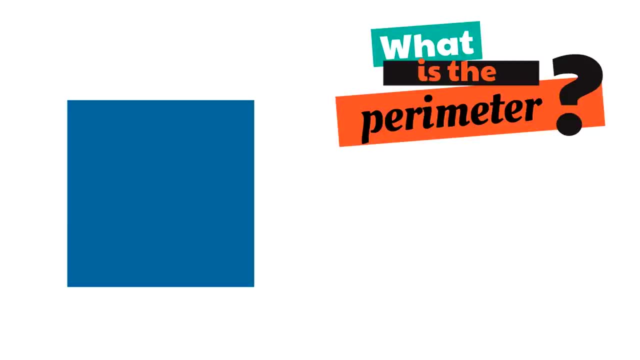 okay, so this is a square, has four sides and all four sides are the same size. Let's pretend we measured it and each side is one yard. Remember, YD is an abbreviation for the distance of a yard. Each side is one yard, Remember. the perimeter is the distance around a shape, so we'll need 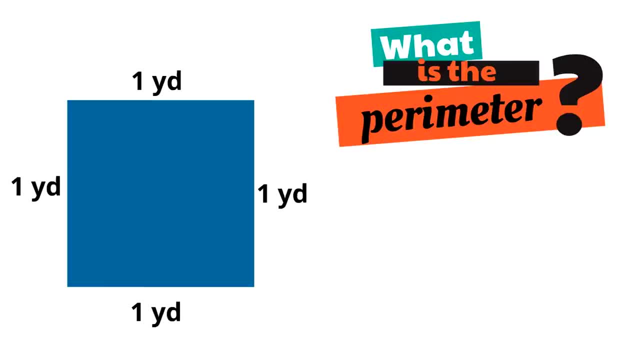 to add all of these sides up. Okay, what's? one plus one plus one plus one? Yeah, four. The perimeter of this square is four yards. The perimeter, remember, is the distance around a shape. If you were to go around this entire square it would be four yards. 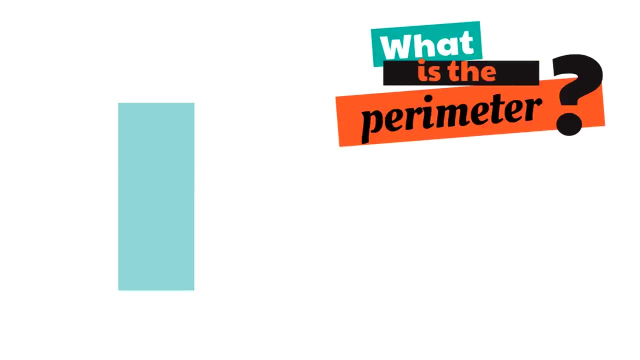 Okay, Okay, Okay. this is the final one. What is the perimeter of this rectangle? Well, first we need to know how long all the sides of the rectangle are, Then we can figure out the perimeter. Remember, a rectangle has four sides, and two of the sides are shorter than the other two. 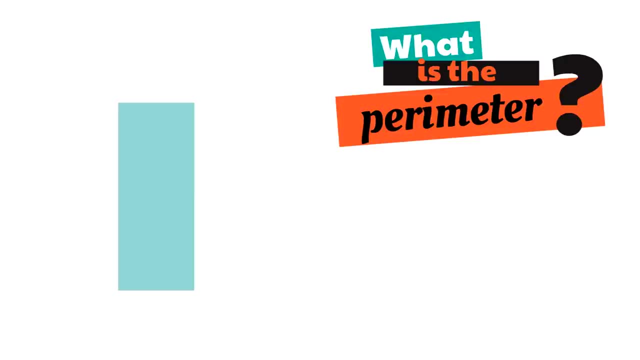 sides With this rectangle. let's pretend we measured it and each side is one yard. Let's add one meter on the short sides and three meters on the longer sides. Okay, remember, to get the perimeter we have to add all of the sides together, so we're going to be adding. 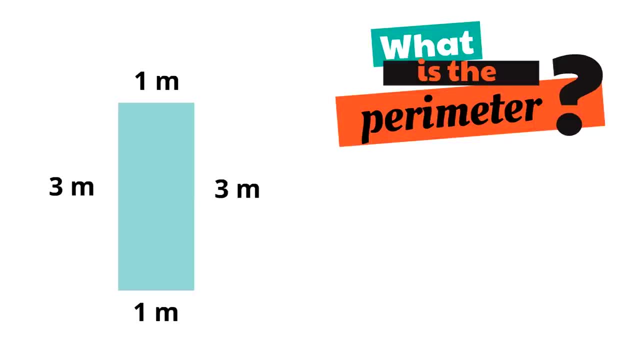 four numbers together. again, To make it easier, we're going to group the smaller numbers together and then put the larger numbers in our equation. What's one plus one plus three plus three? Those are all the sides. What's one plus one plus three plus three? Yeah, eight, That means. 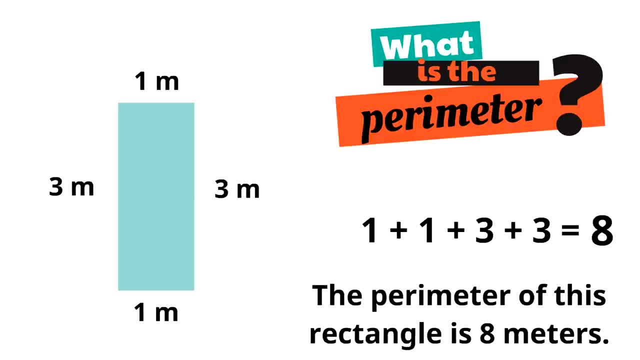 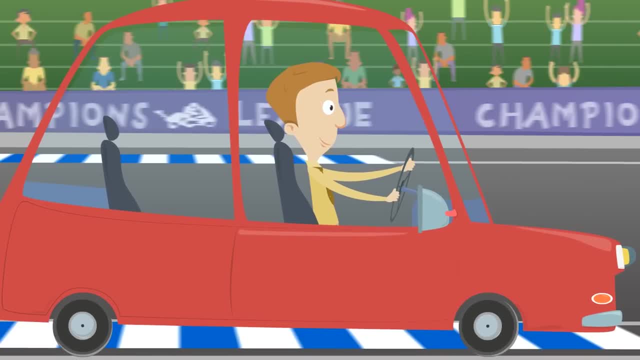 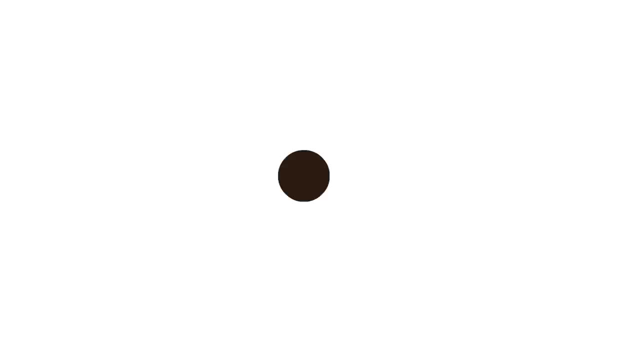 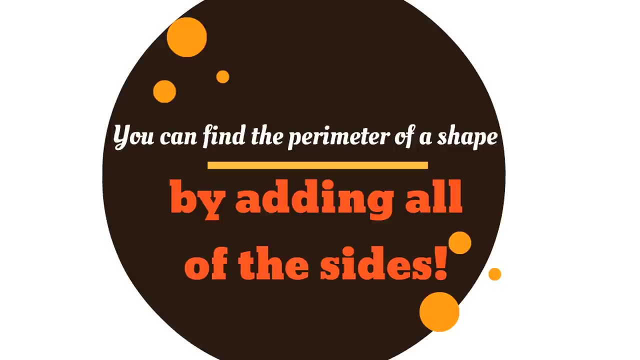 the perimeter of this rectangle is eight meters. Wow, we told you it was going to be fun. Oh, it's such a blast finding the perimeter. The perimeter is so much fun to find, It's like a game. Remember, you can find the perimeter of a shape by adding all of the sides And 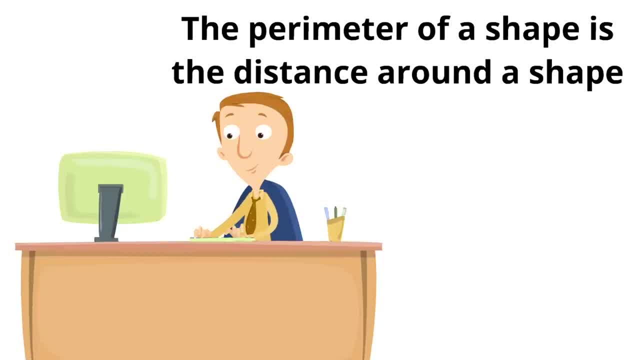 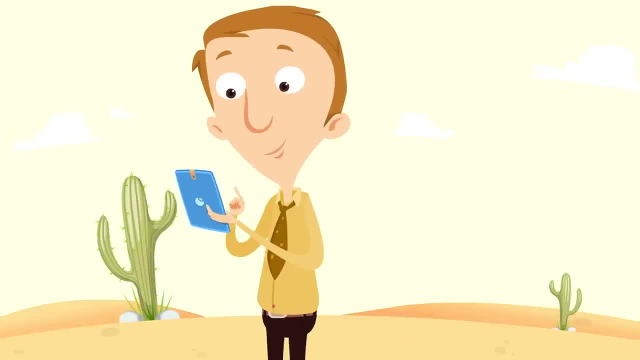 the perimeter of a shape is the distance around a shape. I'm so proud of you. I'm so proud of you. Now you know how to find the perimeter of something. The perimeter is the distance around a shape Of this tablet right? All I would need to do is measure each side and add them together. 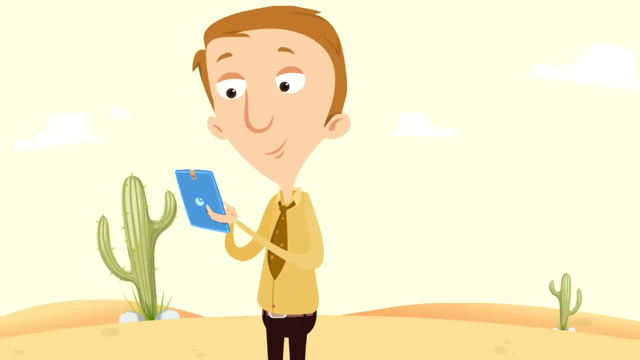 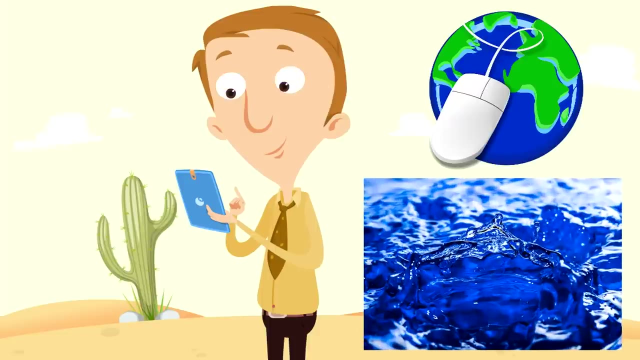 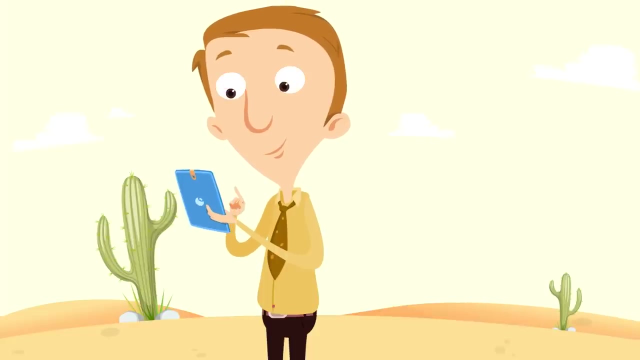 and I would find the perimeter, But right now I got to find an internet connection. There's no Wi-Fi out here. There's no reason to be in the desert. I need water. This doesn't make any sense. Okay, so I'm going to go. You go ahead and find perimeter. Enjoy. The perimeter is the distance. 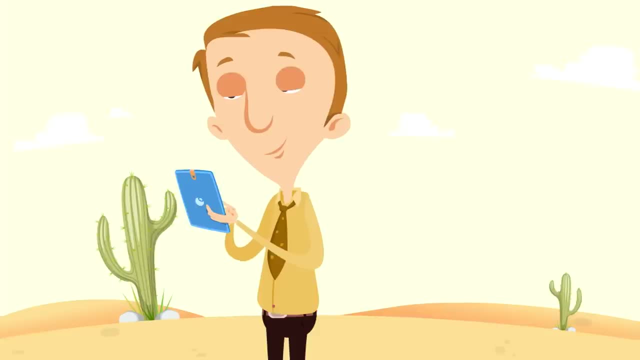 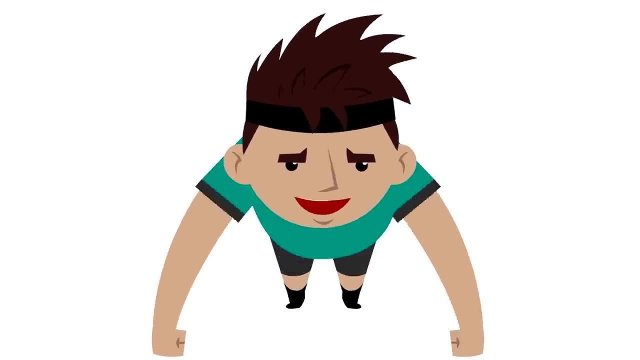 around the shape. Go, Have fun. Thanks for watching. You have been doing a great job, just like Mike, who's doing these push-ups. You know he knows it's important to stay fit and exercise and to stay healthy, And you're like exercising. 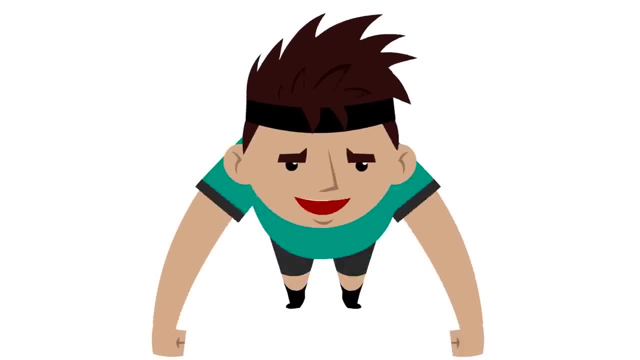 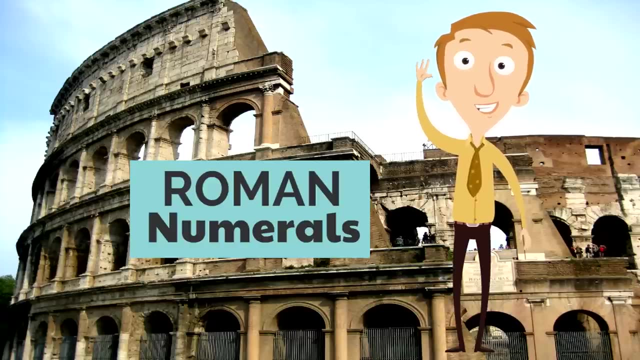 your mind right now, which is super cool, And next we are going to learn about Roman numerals, which is a different way to write numbers, And it was used a long time ago in ancient Rome and it's been used since then And you can think of it almost as a 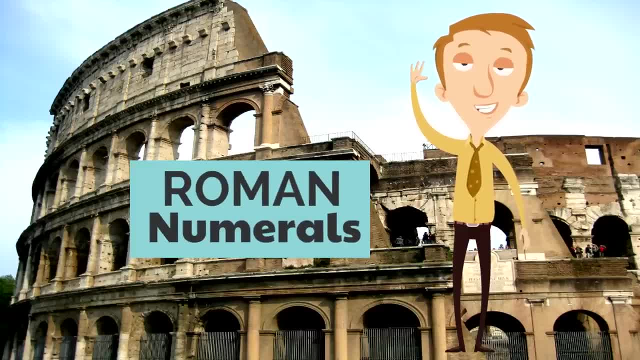 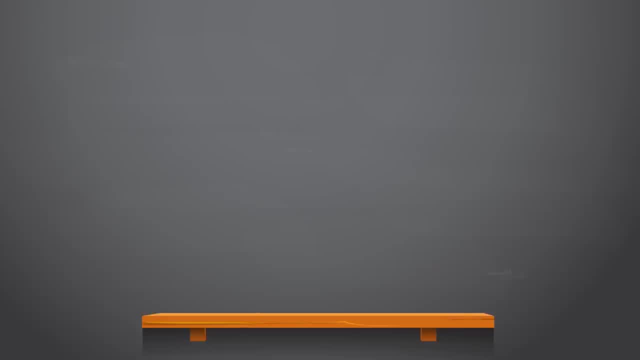 secret code way of writing the numbers. It's pretty simple to learn and we're going to go through that. The first Roman numeral we're going to learn is the Roman numeral I And I is one. I equals one. So if you see an I with a Roman numeral, it's one. The letter V is the. 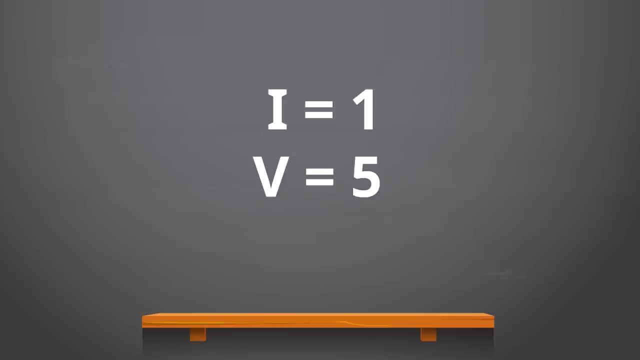 numeral, that means five, And the letter X is the Roman numeral, that means ten. So when you think one, it's an I, If you think five, it's a V, And if you think ten it's an X. So that's it Just. 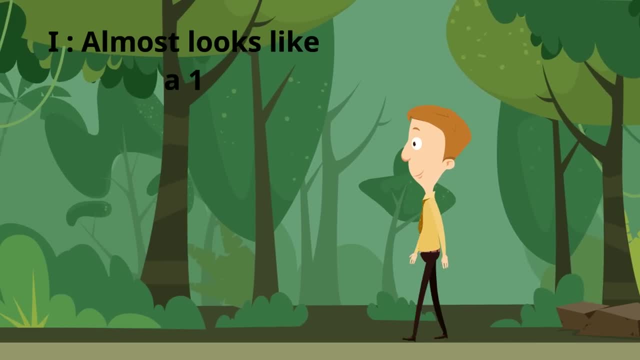 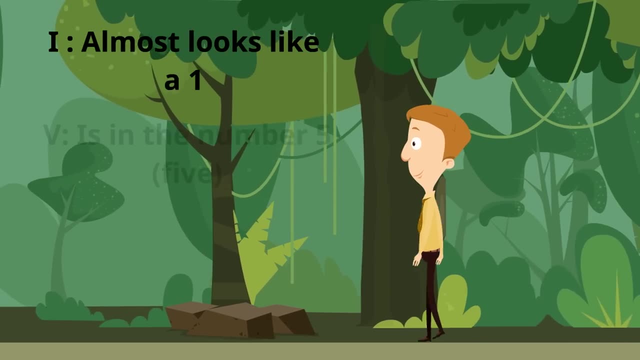 those three? I? it almost looks like a one. That's how you can remember that I is a one. I is the numeral for one. A, V is in the number five. when you spell it out, The number five, you see that. 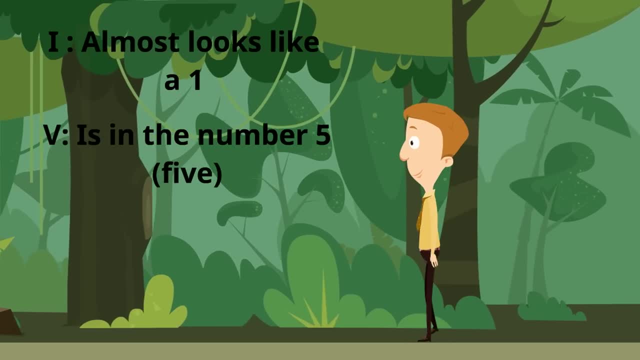 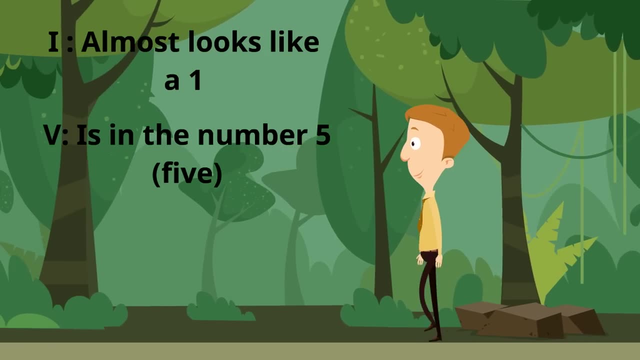 right there, It has a V in it. So when you think of V, you know, oh, you know what? There's a V in the spelled out number five. So V has to be five. Now ten is X And we can't think of anything. 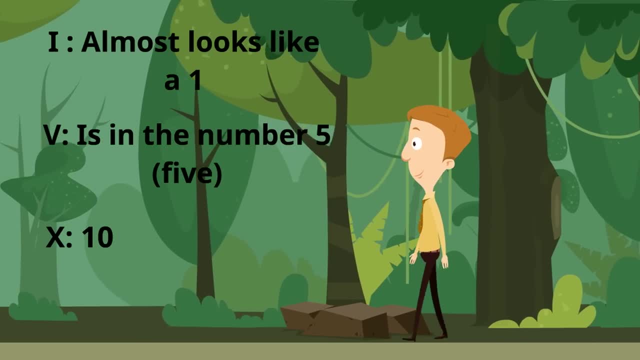 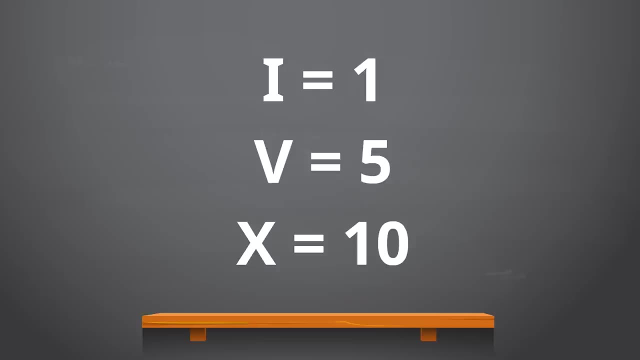 that could remind us of that. So there is no memorization thing. Just when you see the X, it's ten, And that's just what we're gonna have to do. Okay, one last time here. I just want to make sure you get it There's. 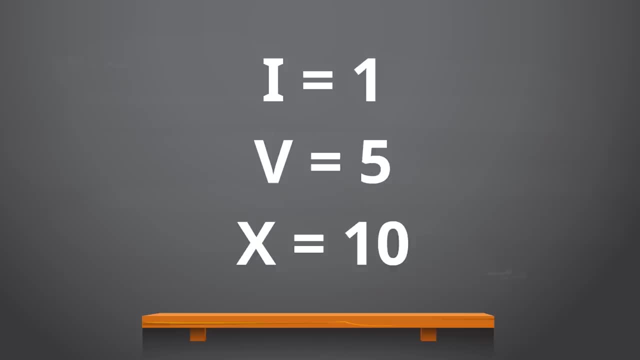 only three. I is the Roman numeral for one, V is the Roman numeral for five And X is the Roman numeral for ten. And you've got to understand that so that we could start playing kind of a game of putting them together and making numbers other than just one, five and ten. So let's get. 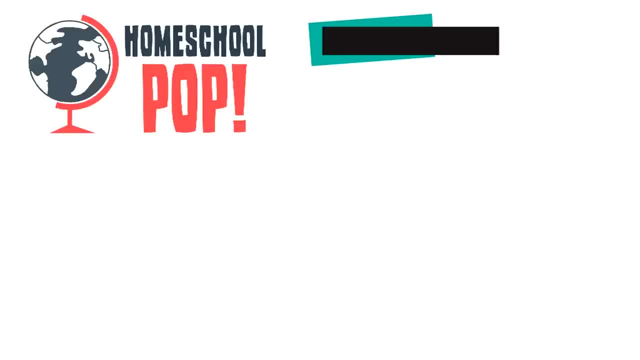 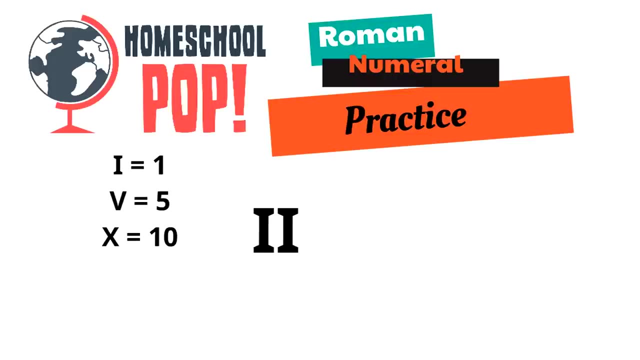 started, So let's practice putting these Roman numerals together. What number do you think this is? You see two I's and I is one, So the answer is two. Two I's is the number two. What about this one? What? 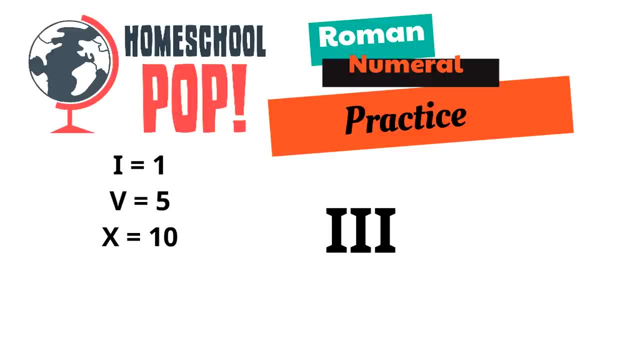 number do you think this is? You've got to guess the number right. There are three I's. There are three I's. Yeah, It's the number three. Let's try this one. What number do you think this is? We see two X's. An X equals ten. So ten plus ten equals twenty. Great job, This is the. 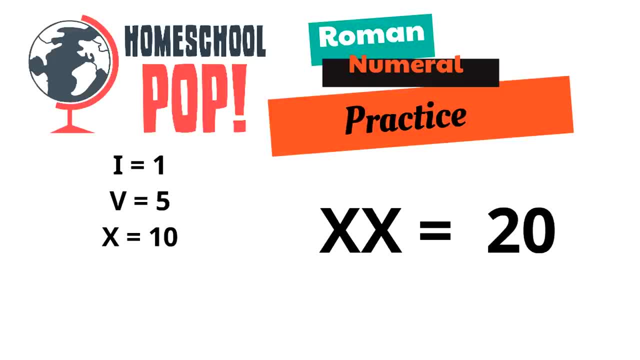 number 20.. Whoa, this one is so cool. Okay, An X and a V. What number do you think this is? The X is a 10.. The V is what number? Five, Awesome. So what is 10 plus 5? 15. Whoa, Thanks. 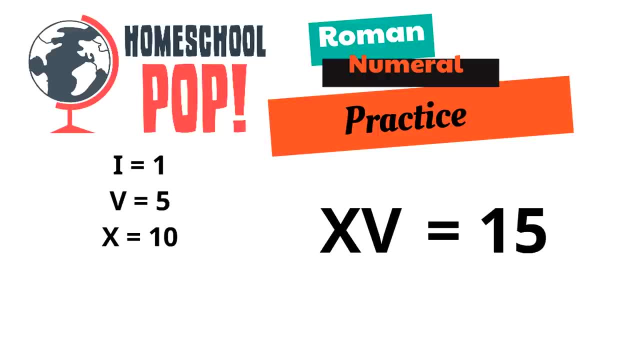 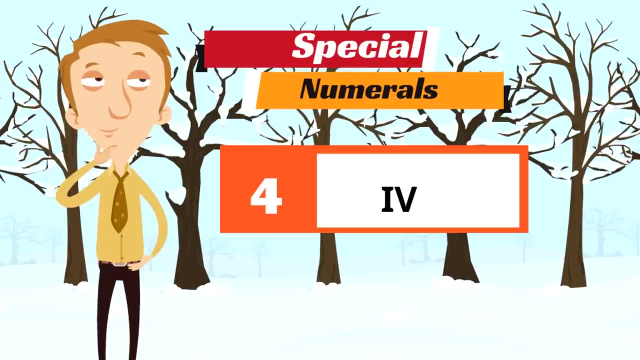 so much for helping out. Now that we've looked at how to put some of these together, I want to tell you about two special numerals that are a little bit different than what you're going to have to just remember these on their own. The first is the number 4.. The number 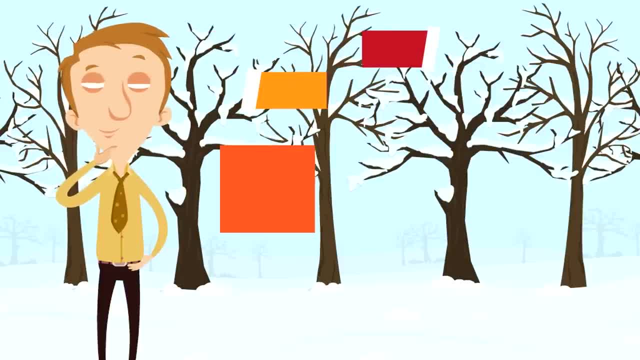 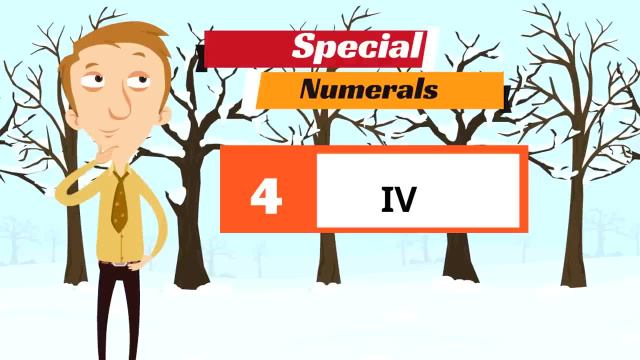 4 is represented with an I and a V. The I is before the V because 4 is one less than 5, which is V. So remember, with 4 it's IV, With 9 it's similar, except with the X, 9 is. 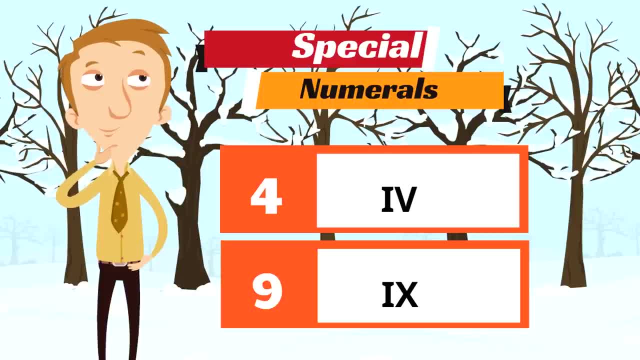 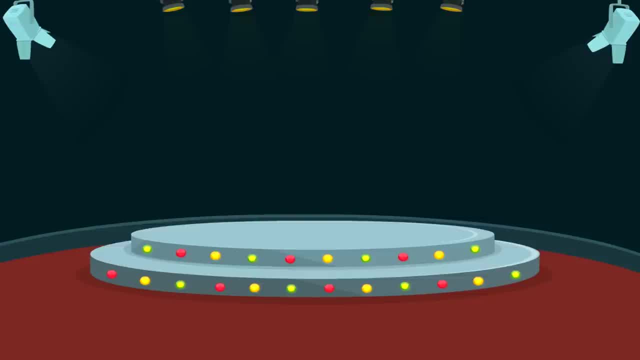 IX. X is 10 and I is just before IV it, So nine is IX. Okay, that was really cool. Thanks for hanging out and learning those with me, But we're not done. We want to go through all the numbers up to 30 just using the numerals And 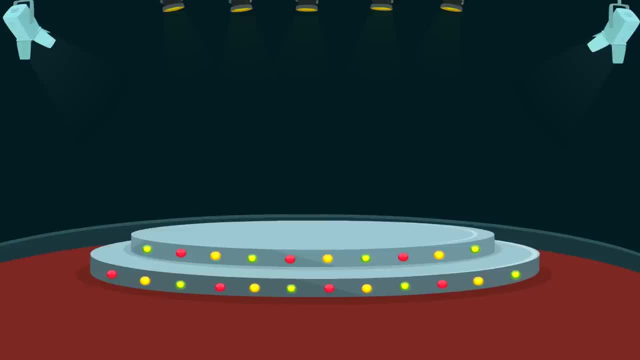 I want to see how much you've really learned. So if you'll do me a favor, as the numerals go up, I want you to say the numbers along with me and we can practice together. Sound good, All right, let's get started. One, two, three, four, five, six, seven, eight, nine, ten, eleven, twelve. 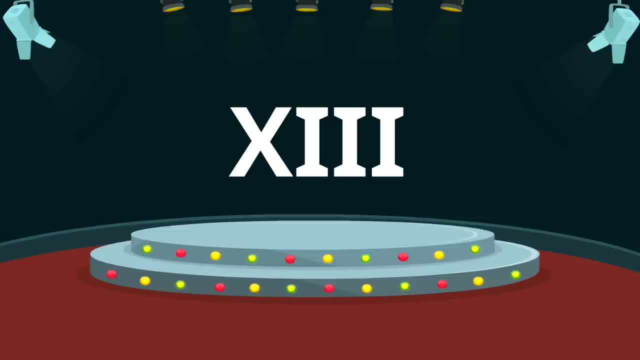